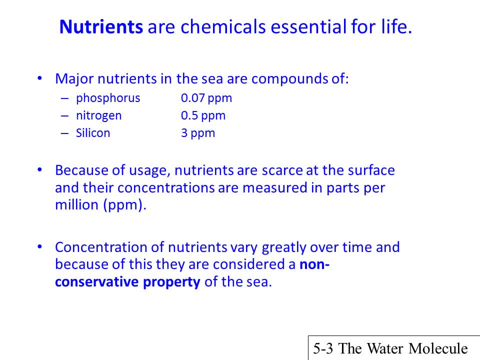 So nitrogen, phosphorus, to a certain extent silicon, which is used for building the shells of little beasties. So these are also inorganic molecules, so nitrates and silicates, And phosphorus or phosphate even, But they're all kind of a separate class of inorganic molecules. 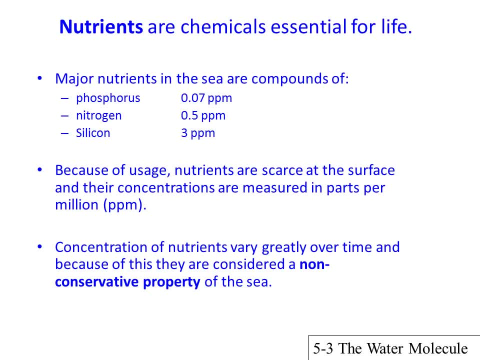 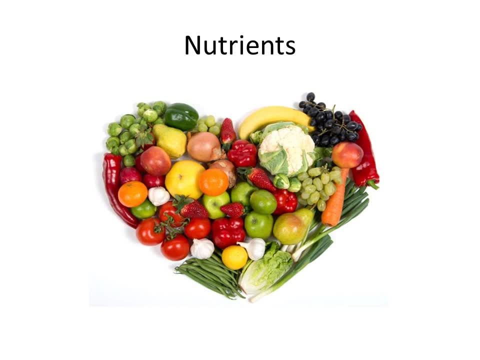 So they're separate parts of what we traditionally call salts and they're really useful in terms of life. So life uses these special elements, these nutrients, to exist. So this is what you get when you Google nutrients. So for all of this biological activity to happen, it has to have these nutrient elements. 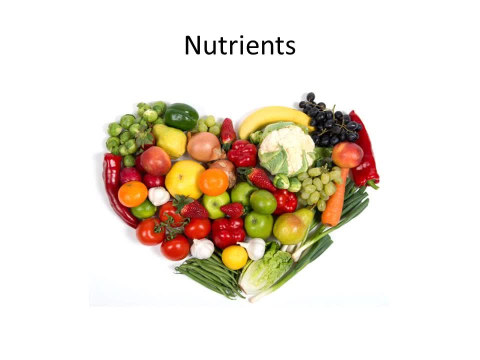 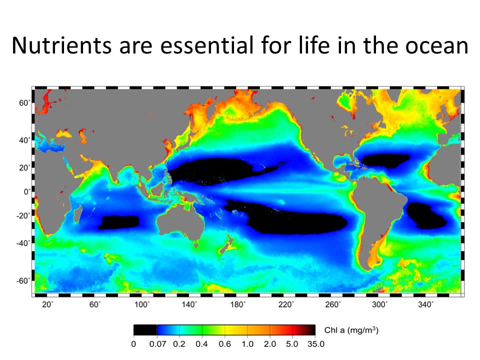 To enable, basically, photosynthesis to happen, a whole variety of biochemical processes require those elements. Okay, so this is just a map of. this is chlorophyll A, So this is basically a map showing where biological activity is going on. 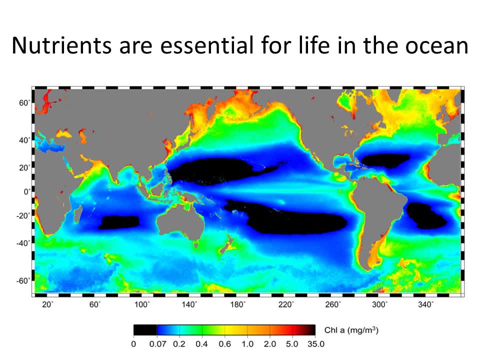 This is a map of how much photosynthesis is happening And you can see that it's not kind of evenly distributed over the whole oceans. It's quite close to end coasts And along the equator. Okay, And the reason for that is these are the regions which are supplied by the nutrient-like elements. 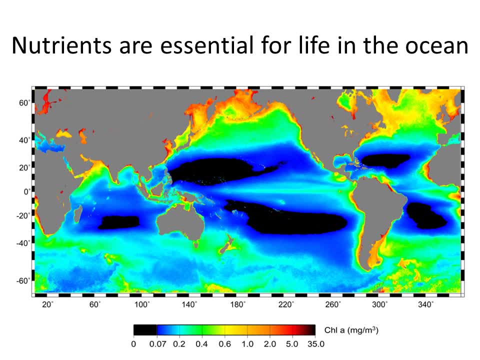 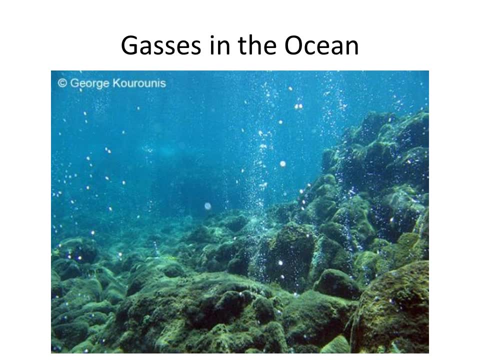 And we'll come on to talk about how that happens in the next lecture, or the next lecture that I give, Because there's some other lectures in between. Anyway, There are also gases dissolved in the ocean, So it's not just dissolved ions. 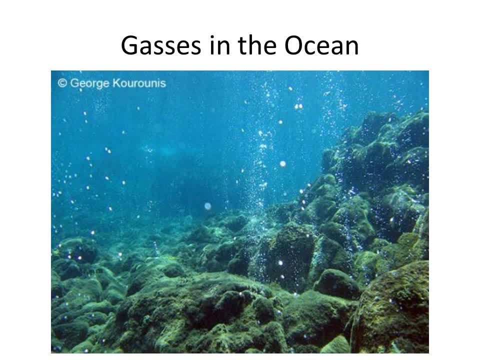 We also have dissolved gases. So this is an image of the seabed, I think in Italy somewhere, And you can see that there are gases bubbling up through the ocean here, because this is on top of a volcano, But there are also gases dissolved in the liquid. 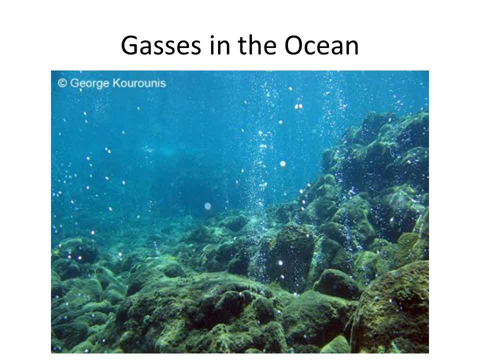 So carbon dioxide is one of the most important of those gases, But there are also things like oxygen, which is important if you're a fish and you want to breathe, But things like also kind of all of the gases in the atmosphere, so nitrogen, argon, all that kind of stuff- are also dissolved in the ocean as well. 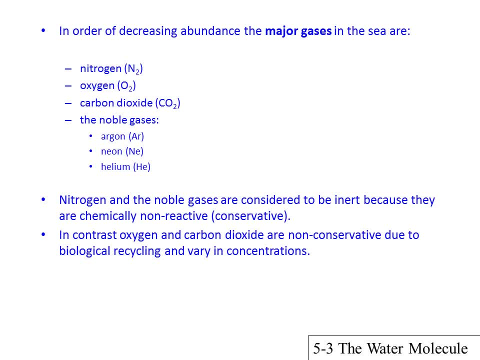 So there'll be electron as well. Okay, so these are the major gases dissolved in the ocean. I'm sure you can read those in your own. Some of them are useful, like oxygen, carbon dioxide. Some of them are less useful, like nitrogen. 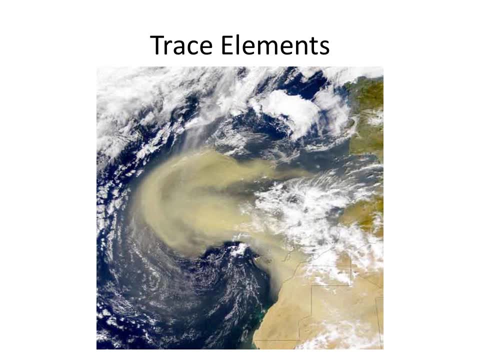 It's pretty inert. And then we come on to these things which we would kind of usually refer to as trace elements. So these are essentially other salt-like elements, but they're only present in very, very low concentrations. Okay, and we'll come on to why they're there. 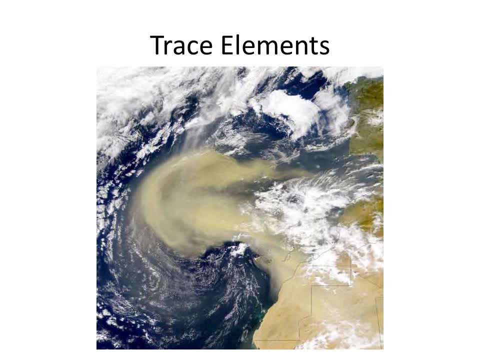 Concentration distributions are slightly different to things like sodium or chlorine, Okay, But these are elements that get added to the ocean, things like this. So this is a dust plume, this is a dust storm in Africa, very dusty continent, And that's blowing out dust into the Atlantic Ocean and that's bringing with it a whole bunch of elements which we usually associate with terrestrial materials, things like iron and aluminium. 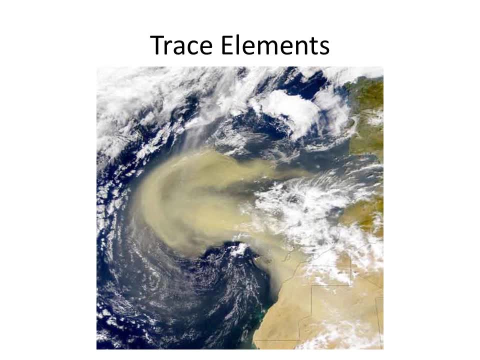 And they're being added to the ocean in very small quantities. Okay, So it looks like there's a lot of stuff being added here, but the ocean is really big. Okay, So this dust plume is actually a very small event in terms. 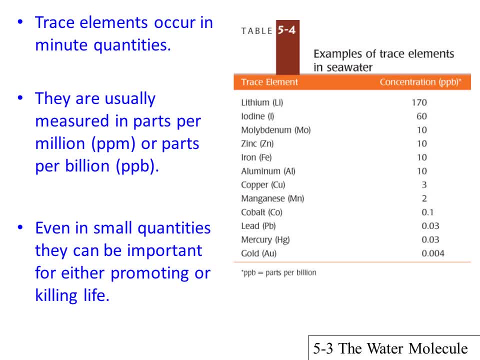 So it looks like there's a lot of stuff being added here, but the ocean is really big, Okay, So this dust plume is actually a very small event in terms of the overall chemistry of the ocean. Okay, And these are some of those trace elements. 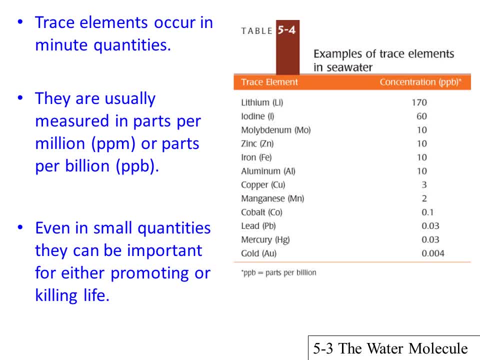 So they're usually measured in things like parts per million or even parts per billion. There are some trace elements which are even lower concentration, So this is one of the elements that I do. my research on Thorium is present in Reactions. 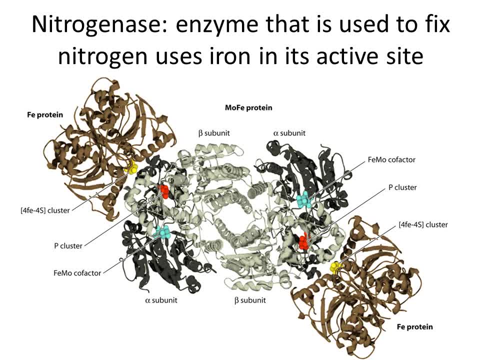 So, for instance, this is an enzyme, nitrogenase, which is important for some biological activity. This is particularly important for the fixation of nitrogen gas into usable forms of nitrate. Sorry, usable forms of nitrogen, In this case ammonium. 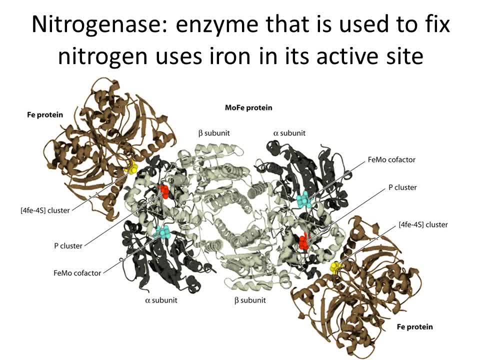 Ammonium, which is converted to ammonium. But this large organic molecule here wouldn't work, It wouldn't fulfill its biochemical function if it didn't have these, These little metal sites. So let's see if I can So these little things here. 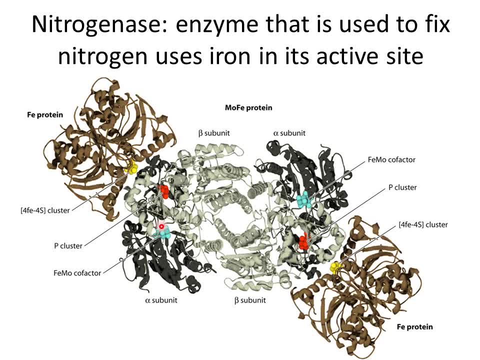 There's a phosphate cluster here And there's a cluster here of atoms that include iron and molybdenum. So these are as far as the overall composition of this huge molecule. it's got many thousands of hundreds of, maybe carbon atoms. 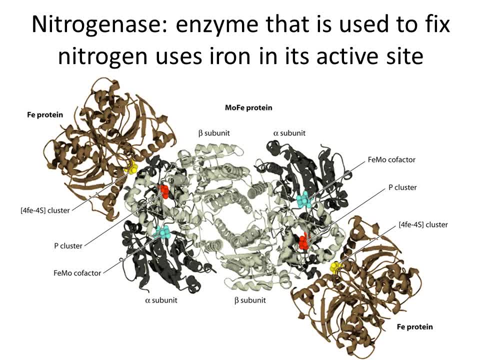 But there's one or two iron atoms that make that molecule do the thing that it does. Without that, Without that iron, you could not, that molecule wouldn't work. Okay, so you wouldn't be able to fix nitrogen in the ocean without small amounts of iron. 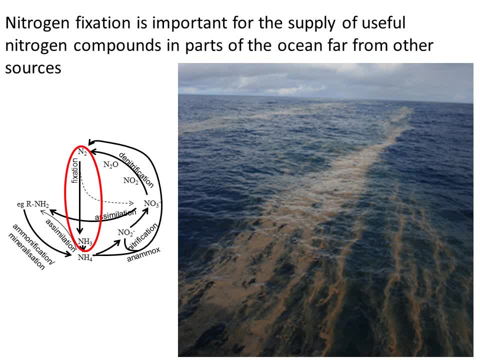 Okay, and this is, this is basically so. this is a. this is a bloom of a kind of a marine plantain called Trichodesmium, And you can see that blooming here. you get lots and lots of these. I mean, this is bazillions of cells floating around in the ocean. 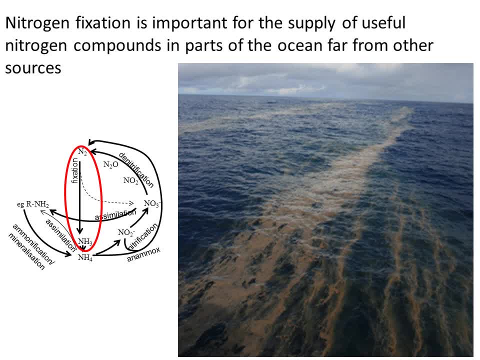 That's why it's brown And it's basically forming that function here which, for those of you that did evolution of the living earth will remember. So the nitrogen cycle has got all these kind of different wacky processes going on over here. 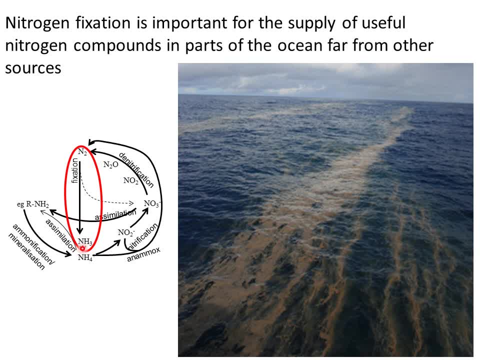 But it's this one that converts nitrogen gas into ammonia and then into ammonium. So this process here is basically driven by that molecule inside these little Trichodesmium beasties, And that molecule only works because of the iron that's there. So so even these things, these trace elements, sometimes referred to as micronutrients- 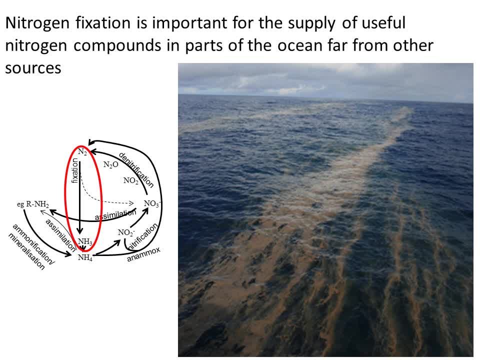 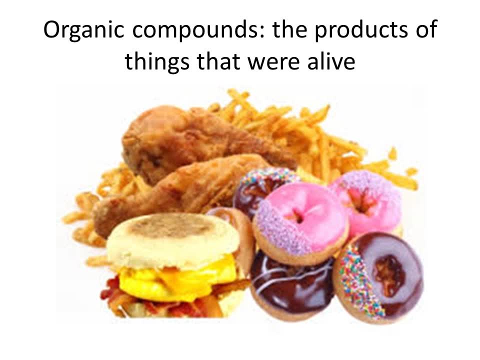 are really important for what goes on in the ocean Moving on, Okay, and there's also, I guess, finally, another class of components, which is basically the organics. So there are some organic molecules that are kind of just dissolved in the ocean. 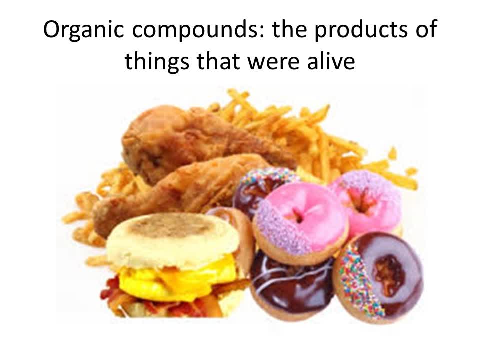 And they're basically the result of bits of things that were living. Okay, so in here we've got like some chicken and some chips and some donuts and a couple of other stuff, But it's basically anything that was alive in the ocean. 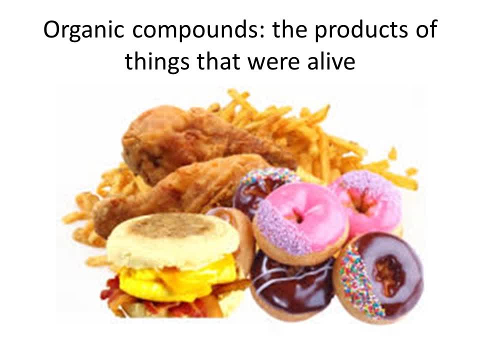 However, that's been processed, either through dying or being eaten or anything that those organisms secrete- those will eventually break down into simpler organic molecules And that organic molecules- that pool of organic molecules in the ocean, forms basically another kind of type of thing that's dissolved in the ocean. 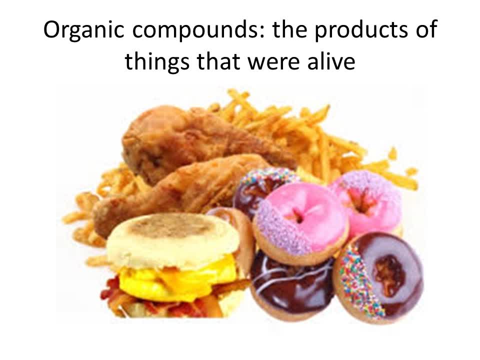 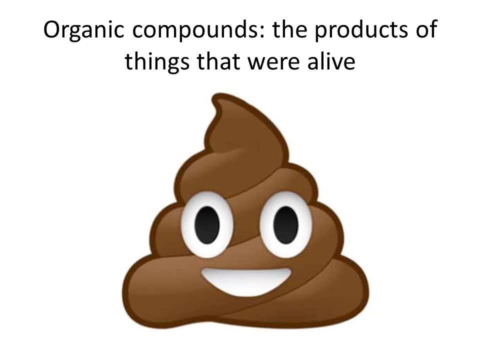 In this case, it's basically a reservoir of organic carbon that could be used for stuff So eaten by other organisms or not. So it's not just things like food, but also things that anything that's been through an animal okay. 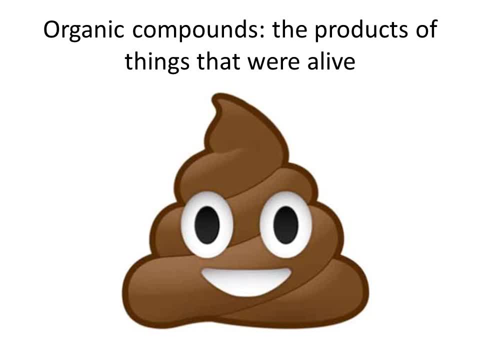 or been through anything that's been living, in this case the emoji of poop, But that's that kind of so anything. so, basically, there's a lot of organic material in the ocean that's been processed through organisms, Okay, and these are all those kind of things. 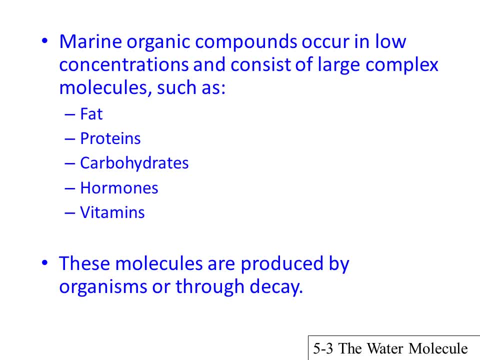 Some of these. so some of these things are, I mean they're naturally occurring. I mean, I guess all of these things that can be dissolved in the ocean can be considered naturally occurring. But in any situation where you add too much of those, 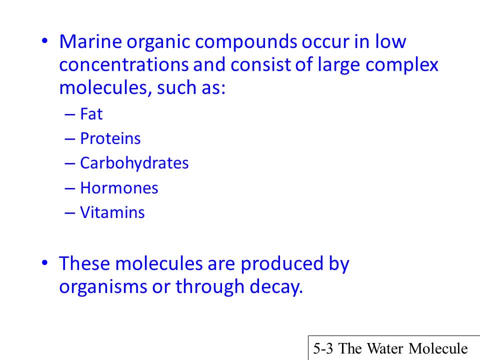 okay, those can be considered pollutants And we'll come on to pollution in the last lecture. So things like too much fat in the ocean can be considered pollutants. If you put lots of fat into a river, that's probably bad. We've put lots of hormones into the ocean and into rivers and stuff like that through contraception. 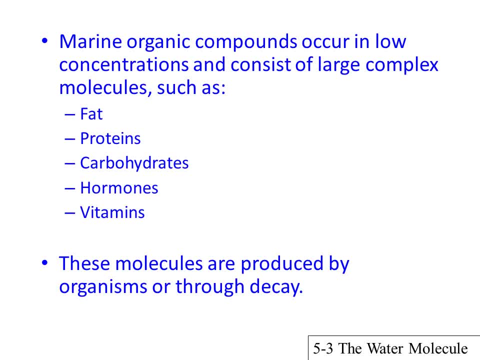 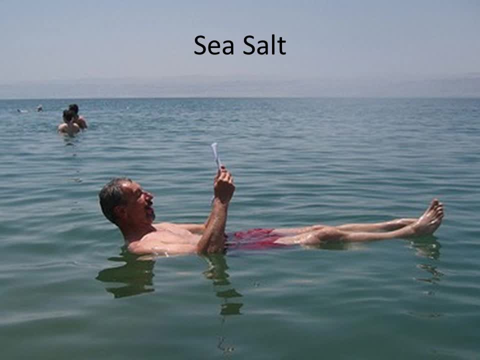 So there's lots of oestrogen whacking around in the environment, which is pretty bad if you're like a fish. Anyway, but the rest of well, most of this lecture, we're going to talk about sea salt. 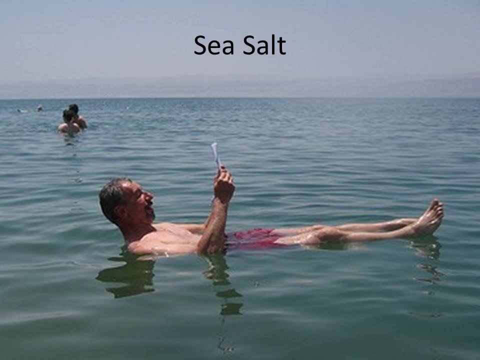 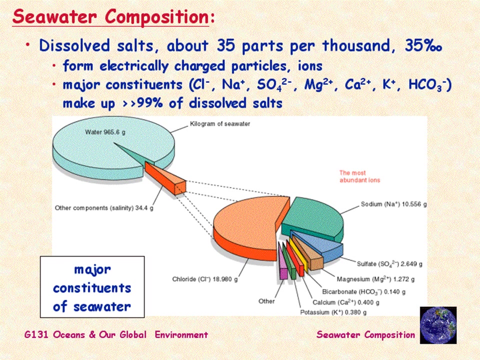 So this guy here is floating in the Dead Sea because there's lots and lots of salt dissolved in it. So this is not the ocean. this is the Dead Sea in Israel slash Palestine. So we're going to talk about sea salt. So sea salt, approximately 3.5% of the mass of seawater. 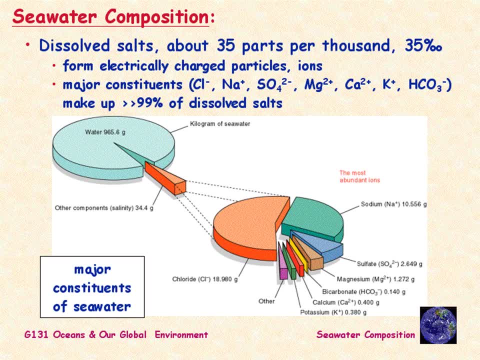 is these dissolved in the organic iron sea salt. So we sometimes see this referred to instead of using percent. quite a lot of the time in genes, The way science is, we use this term here per mil. So instead of this, this is parts per thousand rather than parts per hundred. 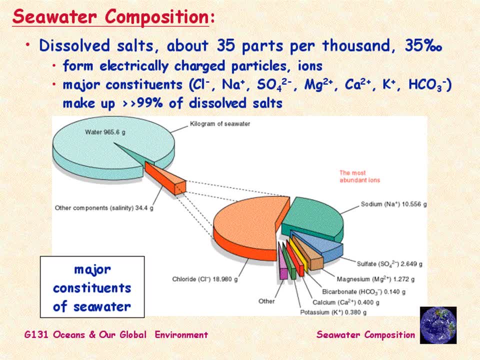 So it's got this little extra zero on the bottom here. So 35 per mil of the mass of seawater is the salts And you can see broken up down here there are a couple of things that it's made of, So mostly chlorine sodium and then some of these other guys here. 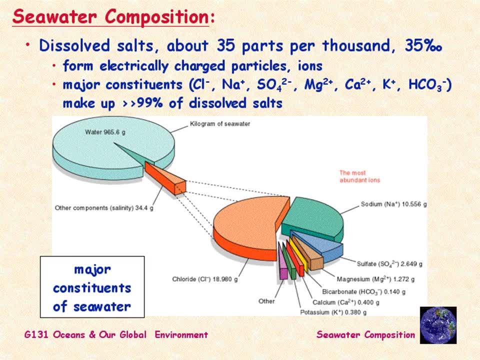 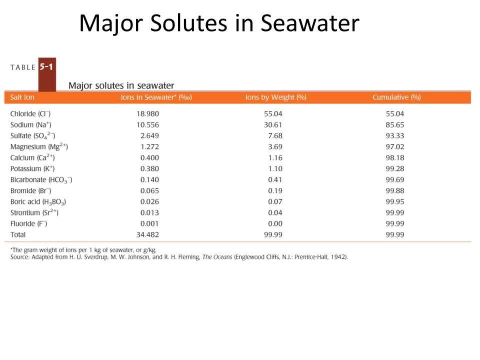 So sulfate, magnesium, calcium, all those kind of goodies, Okay, So that's what it's made of, Okay, And this is the type. So this is the table of that, which I don't expect you to read right now. 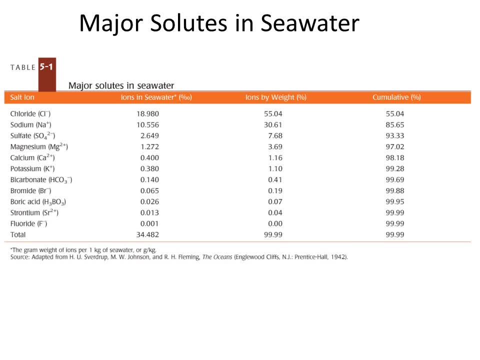 but you can see that. you know, the percentage of ions or the per mil of ions is not the same as the weight, because different ions weigh different amounts. Okay, Just be aware of that if someone asks you a question about it. But where does this stuff come from? 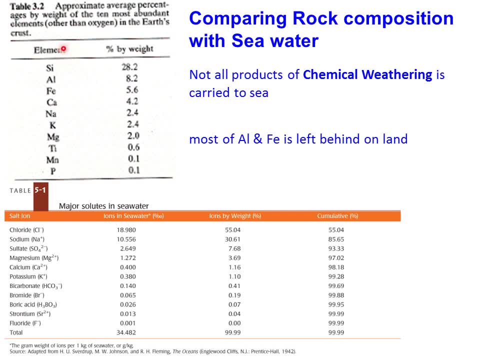 So at the top here, this table up here, is the, I guess an approximation of the average composition of seawater. So this is the table of that, which I don't expect you to read right now, but you can see that you know the percentage of ions or the per mil of ions. 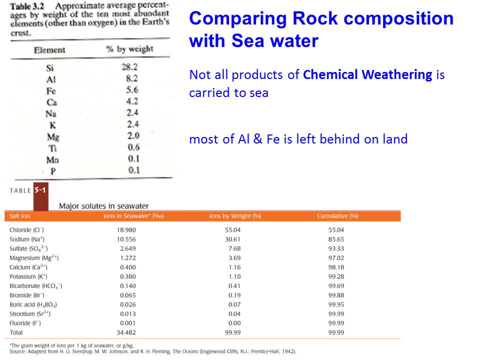 is not the same as the weight of the rocks of the continental crust, And you can see up there that it's mostly silicon, aluminium, iron, okay, Stuff, that's. you know, rocky kind of blah, rocky kind of elements. 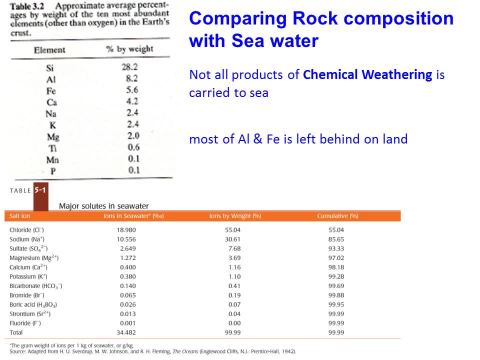 But the stuff in seawater, that's not that Okay. So it's not. we're not just weathering rocks and putting those into the sea. Other things are happening to preferentially allow different elements into the sea and keep other stuff behind. 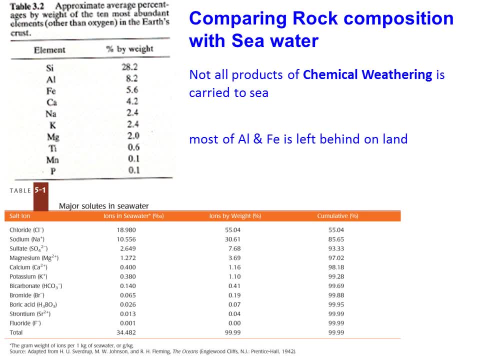 Okay, And in this case we can see that iron and aluminium are not really weathered out from the um rocks into the ocean, And that's because those elements are not very soluble in river water. Okay, So if you weather the rock, the rock is completely gone. 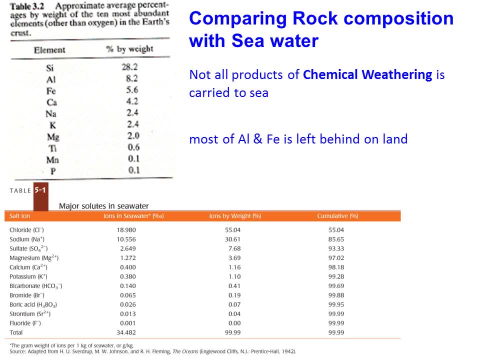 Um, all of that stuff must end up in solution at some point. But the iron and the aluminium don't really make it all the way to the ocean. They quite often get precipitated out as secondary minerals. um, uh, that, uh that get trapped in, kind of trapped in rivers. 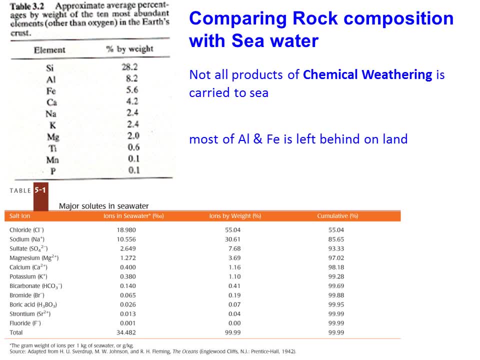 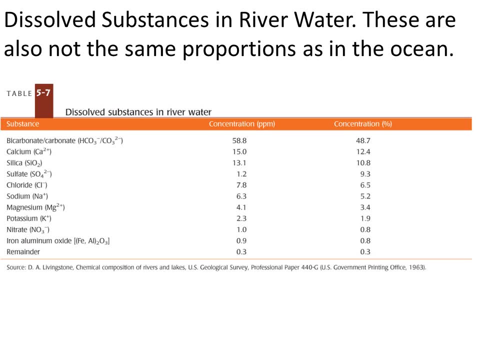 trapped in sedimentary basins, trapped in estuaries, trapped in the coastal environment. They don't make it into kind of the dissolved pool of elements in the ocean, Okay. So that's kind of like that what that says. 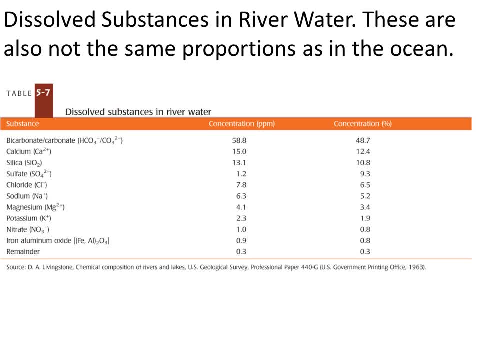 Okay, So this is the. this is the composition of river water. So we can see that the composition of river water is a little bit more like the composition of the ocean. Okay, So it doesn't have the iron and aluminium, but it still has other stuff in it. right? that's not really in seawater. 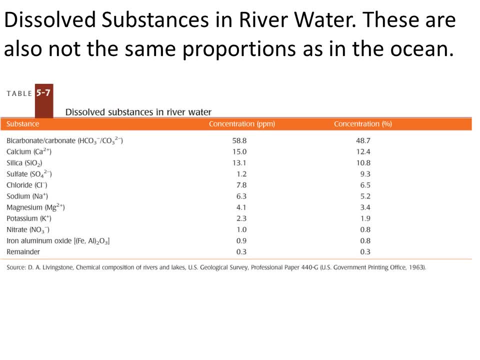 So the um, it has quite a lot of silica, It has quite a lot of bicarbonate, quite a lot of calcium, not much sodium and not much chlorine. Okay, So we have to think about where is the ocean actually getting these other these where it's kind of its composition of salt from? 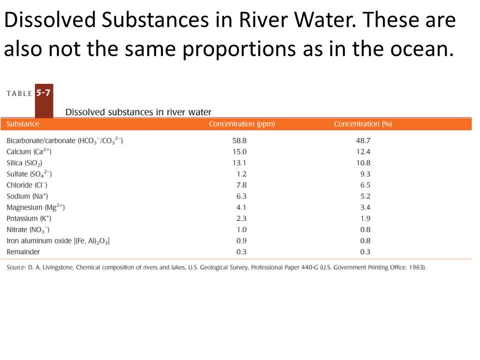 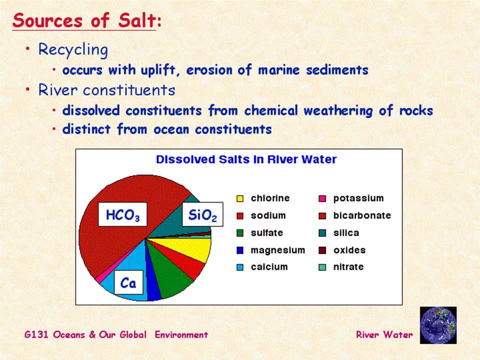 if the composition of the stuff that's flowing in from the land is not the same. Okay, So that's a bit of a puzzle. Okay, So these are. this is a back table, described as like a little picture thingy. 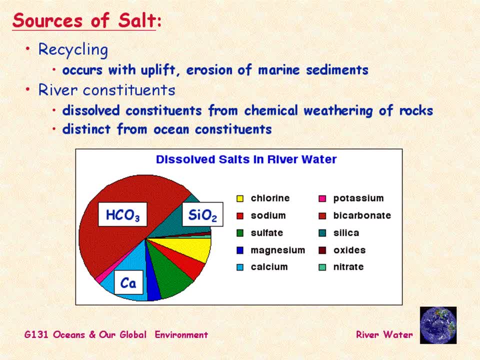 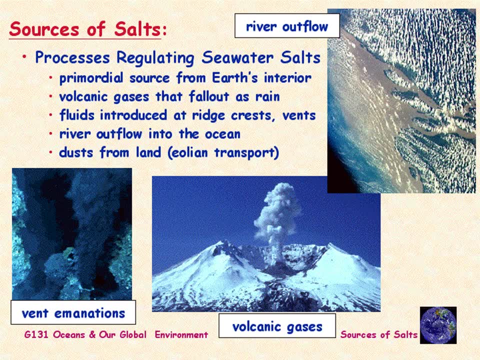 Pie chart. It's not science, This is a pie chart. Um, so this pie chart here. Um, so this pie chart here. Hopefully on the next slide I'll have um. so there are, um. so that pie chart doesn't look like the first pie chart. 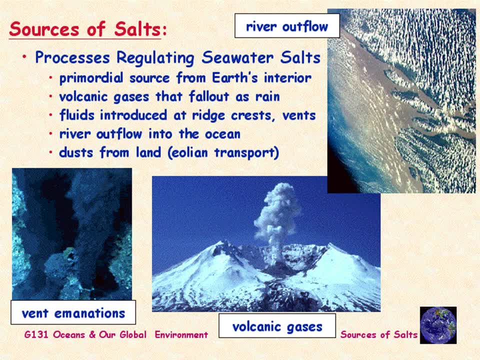 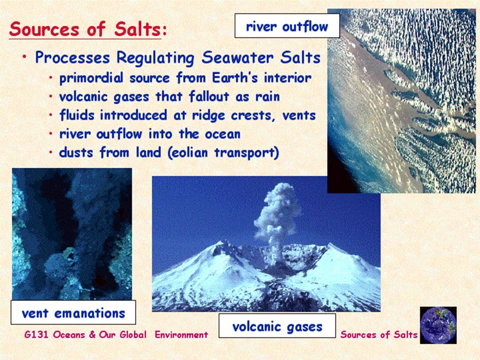 Okay, So it had the ocean and the rivers different compositions. So there are these other places where we could be thinking about where the ocean gets its dissolved salts from. Where does it get all these ions from? So, other than so, up the top here, this is kind of a depiction of, uh, this guy up here. 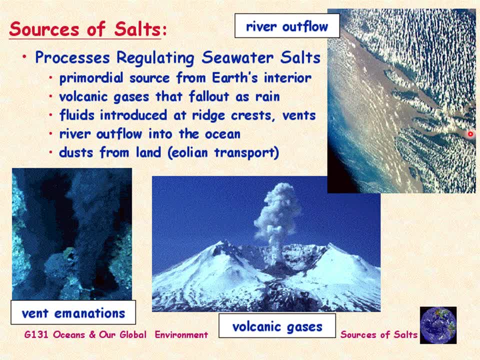 This is a depiction of, uh, what's coming in in rivers. This is, uh, a river and this is some sediment coming out, But uh, so that's bringing elements into the ocean. But there are these other sources as well. 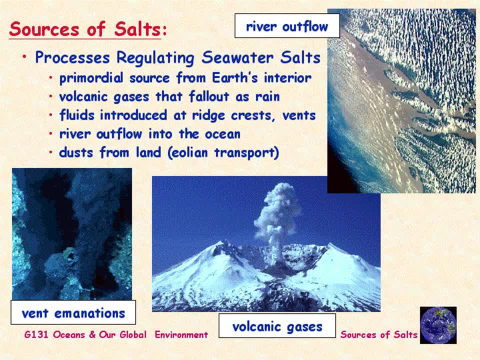 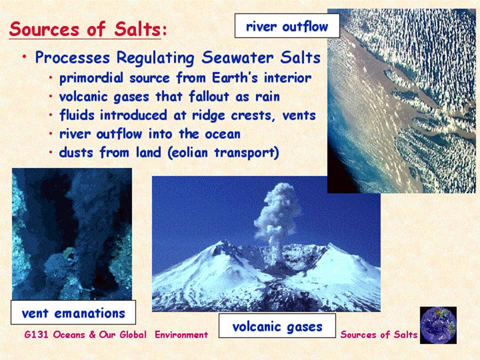 So, uh, vent emissions. So these are. this is basically stuff that goes on interaction with seawater, with underwater volcanoes. Okay, So this is the the content: the oceanic crust interacting with seawater, And then volcanoes on land and in the ocean. when they erupt, they they also, um, give us lots of goodies. 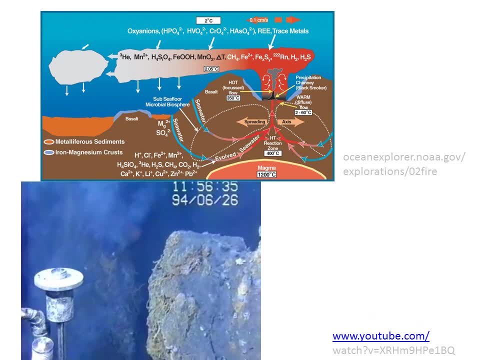 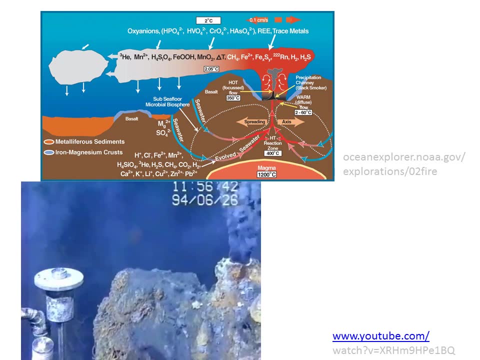 Um, So hopefully this will play And we'll see. Okay, So we can see here that this is a. this is an example of a hydrothermal system. So we've got the uh, something like a, a mid-ocean ridge here. 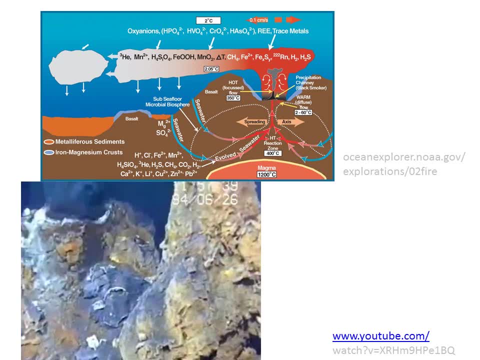 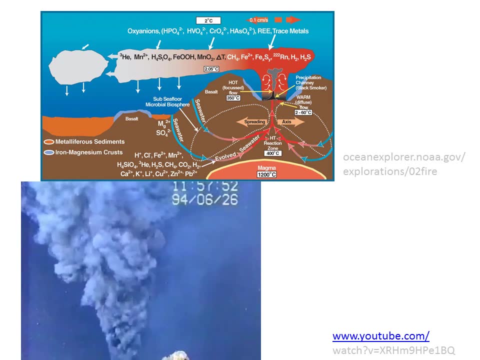 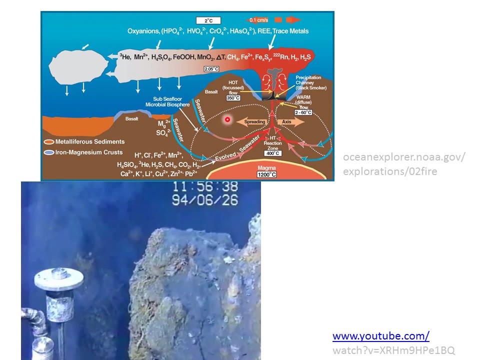 And all of the brown stuff that's basalt rock. Uh, and what happens? is there that we're not directly taking uh elements? Uh, we're not directly taking elements from down here in the mantle up into the ocean. What happens is this? this part of the crust here is very hot. 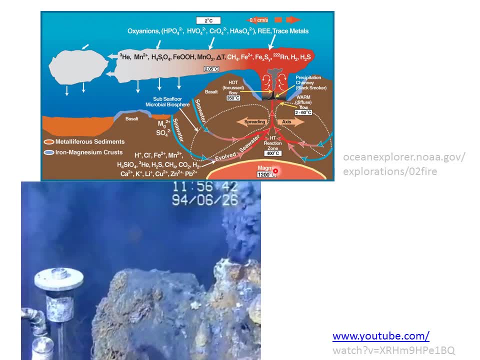 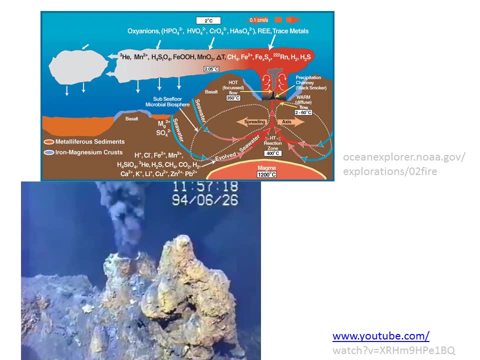 Okay, So there's a volcanic activity going on there. It's quite close to the mantle, So that creates basically the water in that rock heats up, expands and comes out at these kind of smokers down here. Do you see those smokers again? 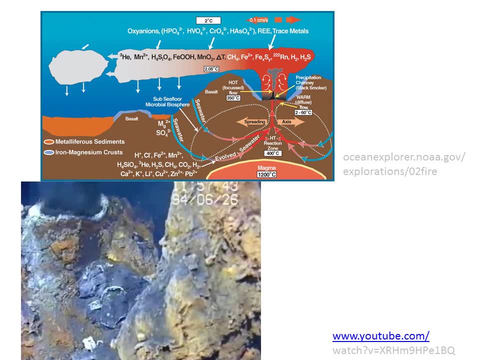 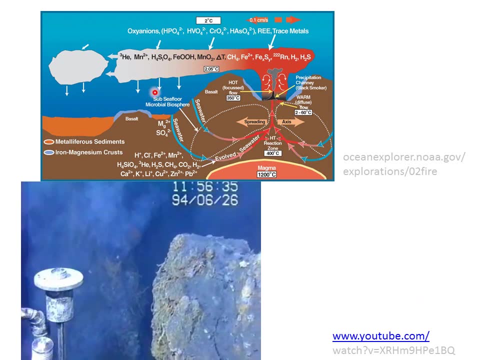 These are black smokers that form on these mid-ocean ridge kind of hydrothermal sites, And seawater then recirculates through this hydrothermal system. So seawater comes through here. It basically leaches the rock Okay, So it doesn't completely weather it. 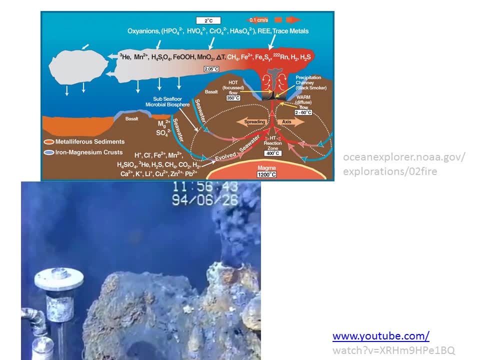 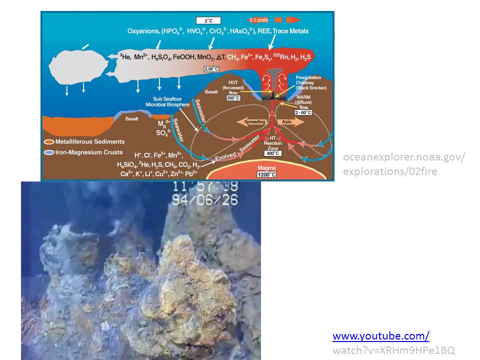 But it's it. basically. you have a high temperature Fluid that goes through that And it strips out some of the elements. So it strips out the elements. It strips out iron, It strips out some chlorine, It strips out magnesium. 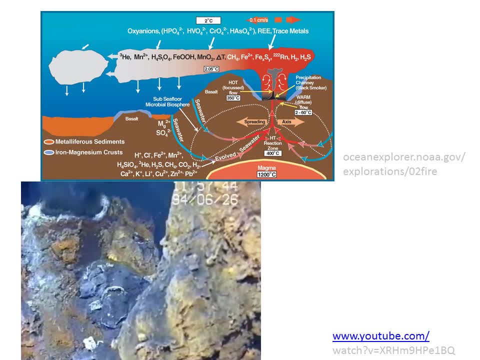 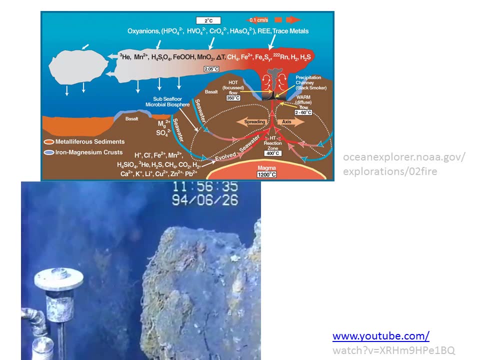 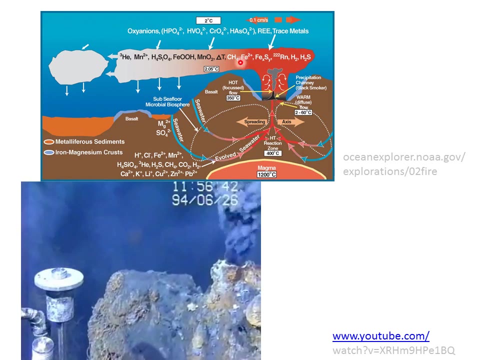 Those get stripped out and added to the ocean. Okay, Now, some of those elements don't really like being dissolved in the ocean, Like iron for instance, And they precipitate straight back out again And, uh, so these, these sediments here are basically. you have basically insoluble elements being pumped into the ocean. 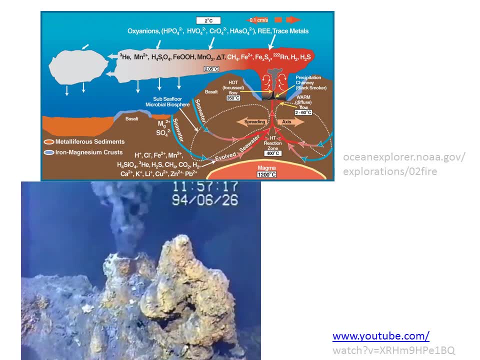 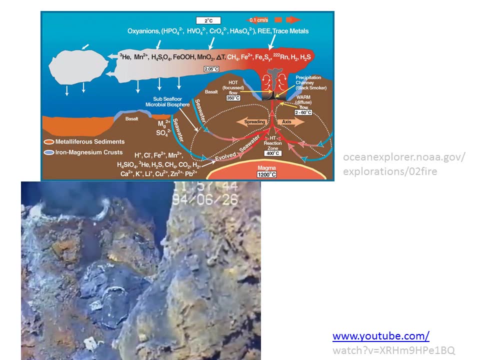 And then they precipitate out again. Okay, And that's where we get, uh, quite a lot of our metal deposits, So like copper ore deposits and things like that, are formed, But it, but it does mean that some stuff that doesn't precipitate out adds to the pool of salts in the ocean. 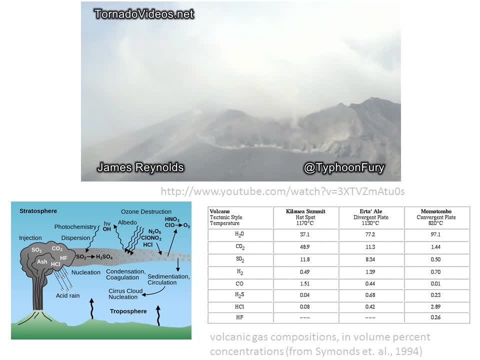 Okay, And moving on to the next, Okay, The other. Okay, so this is this is a slightly longer video, But but the other, the other source of um, of, of particular elements like chlorine And fluorine. uh and sulfur are added to the ocean. uh through volcanic activity. 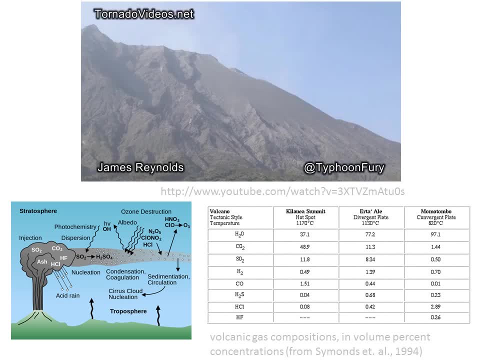 So this is uh, this is some, some pictures of some volcanoes erupting. And those volcanoes are erupting because there are gases that are held in the magma, Either uh recycled through a seduction zone or primary kind of melts from the mantle. 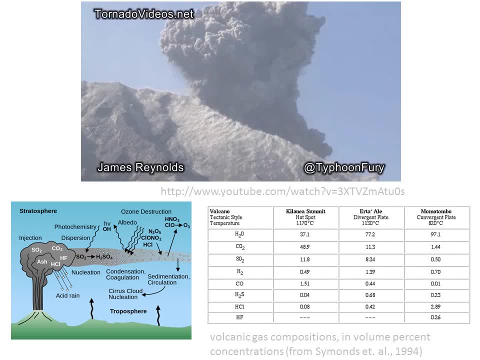 Contain a lot of gases, And those those gases are expanding and causing the explosions. But once they've expanded and caused the explosions, those gases are there in the atmosphere. Okay, So volcanic gases include mostly carbon dioxide, uh, sulfur dioxide, things like that. 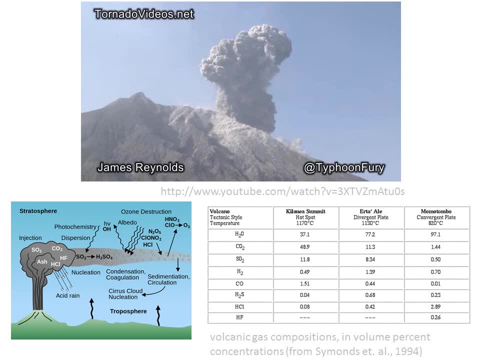 Which you might have covered uh a little bit in ELE from their climatic effects. But there are also other gases in there as well. So hydrogen fluoride, hydrogen chloride And those uh gases uh precipitate out, eventually uh through acid rain and go into the oceans. 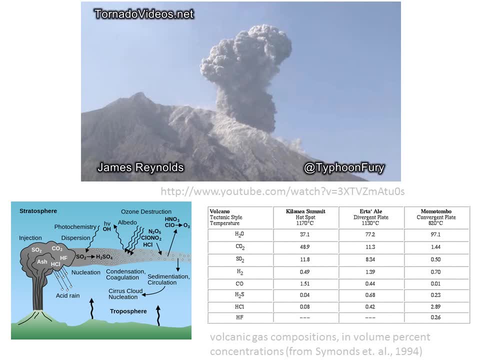 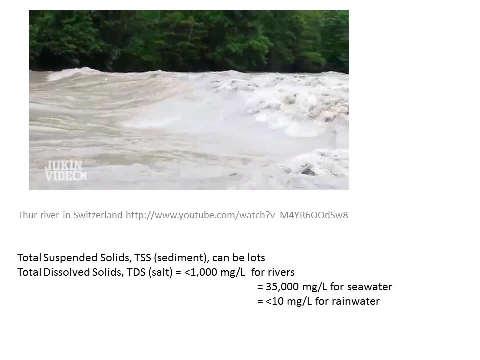 So Most of the chlorine in the oceans comes from a process like this: It goes through the atmosphere and down into the ocean. Okay, So the last, last little video is looking at the river flux. So this is- uh, this is the river somewhere in Switzerland. 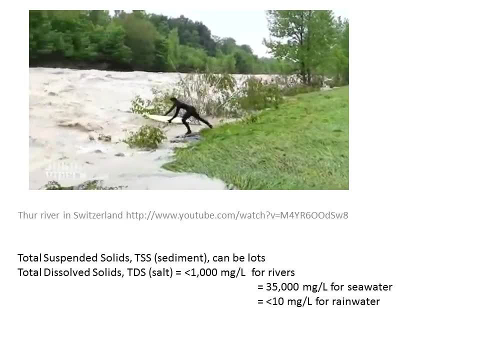 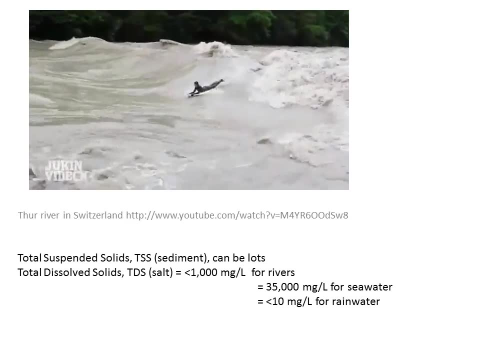 You guys um, surfing, Um and I, and basically the. the point of this is to say you can see the river. There's quite a lot of stuff in the river. Okay, It's quite mud, Yeah, Uh, you might see some trees that I passed by. 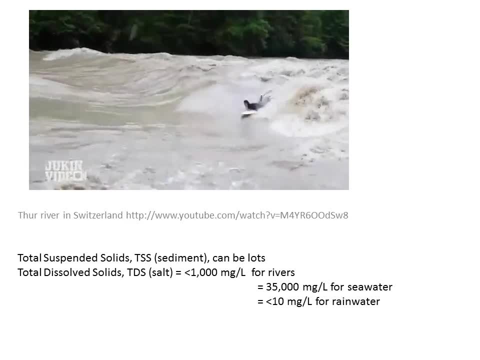 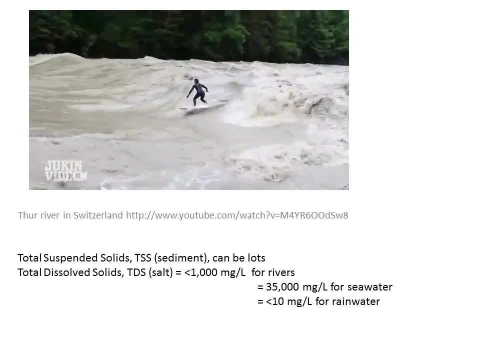 Um, but there's lots of stuff in the river, But it's not just the stuff that you can see. The stuff that you can't see is the total dissolved solids: Um so, Um, But there are these, uh, Okay. 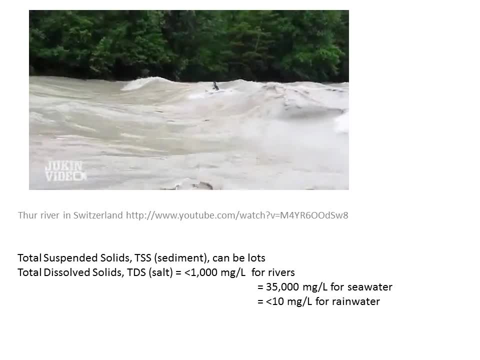 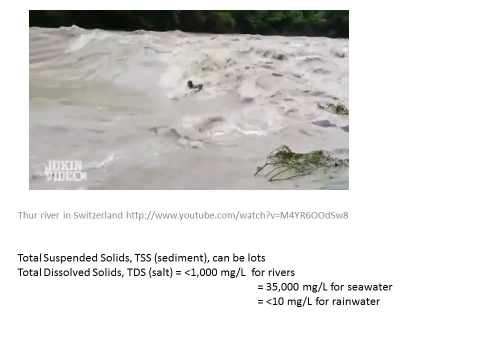 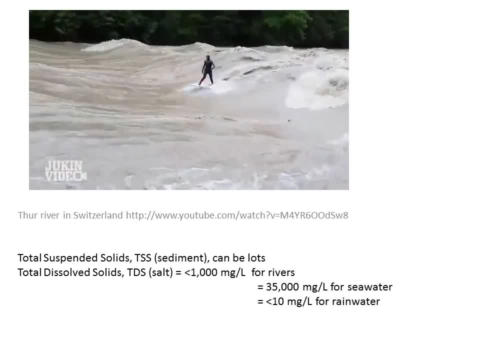 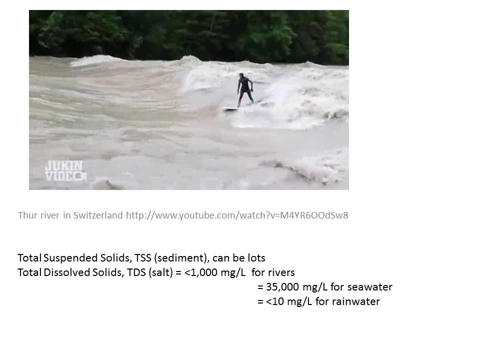 Yeah, Yeah, Yeah, Yeah, Okay, Uh. so, um, In addition to all of this stuff going down this river, there is some dissolved material. Okay, And girls can surf as well. Is there a girl surfing? There we are. 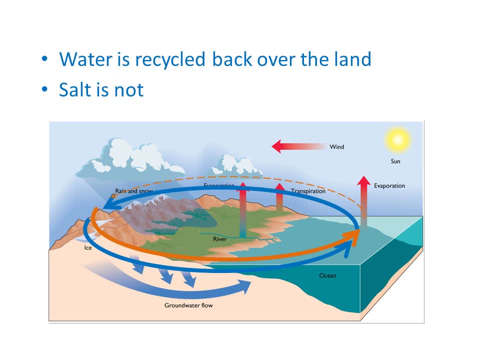 And See how she does. Okay, So, uh, at the end of last my last lecture, uh, we talked about this. why the, the, the ocean was salty. Okay, So, all of these things that are being, all of these sources. 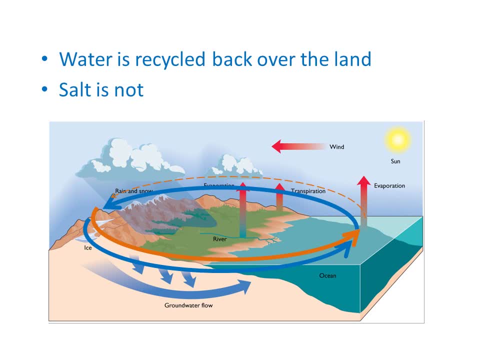 Okay. The rivers, The volcanoes, The hydrothermal activity, The ocean, The ocean, Okay. So all of these things that are being all of these sources, okay. The rivers, The hydrothermal activity, they're all adding salts to the ocean, okay. 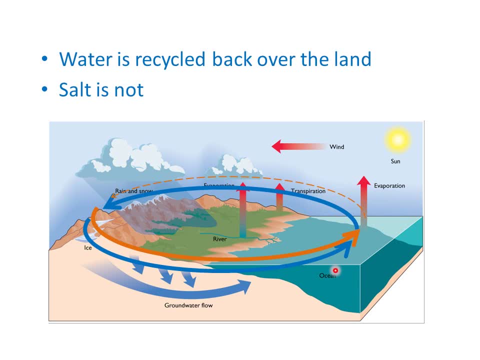 So they're all adding goodies into our ocean here, But when that water evaporates, okay, only the water is evaporated back over the land. okay, A small amount of salts comes back. So we do get like sea spray back from the ocean onto the land. 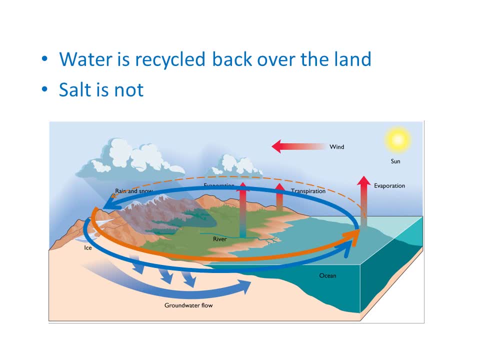 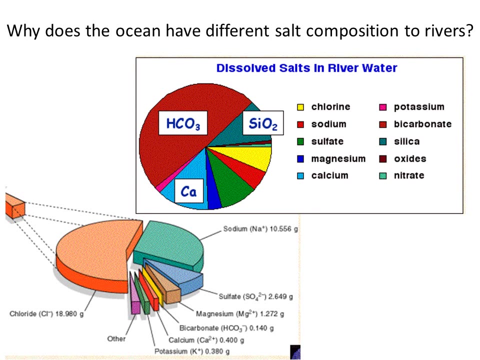 If you know, after it's been particularly stormy, if you lick a car it's a bit salty. I mean, don't lick a car, but you know, So don't do that. Okay, so we've got this. we've still got this conundrum that. 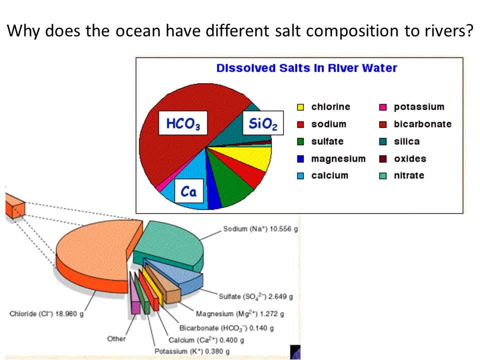 although we've got all these different sources of salts to the ocean, the ocean is a very different composition to the sources. okay, So things like, particularly things like chlorine and sodium, they're not added at the same rate that all of the other stuff is added. okay. 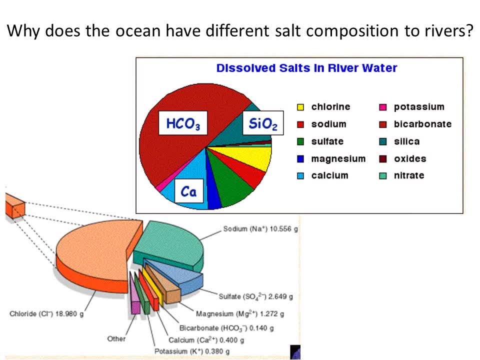 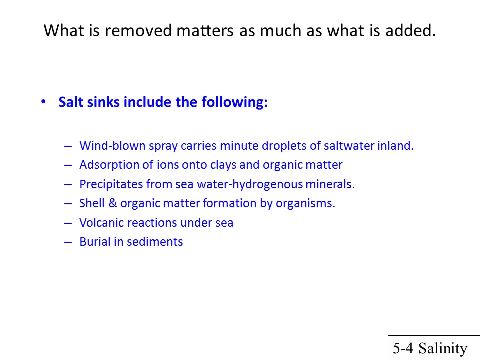 So if we just summed up all of the sources and did that recycling of water, okay, we still wouldn't get the same composition of salts as we have. Okay. so it's not just what's added to the ocean that matters, it's also what we take out, okay. 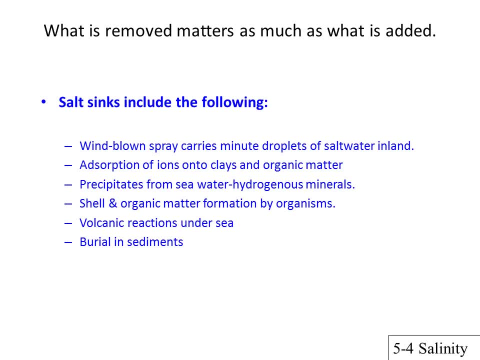 So that what I mean if you have, basically if you have a bucket of stuff, the composition of that your bucket of stuff depends on what you add to that bucket but also what you take out. okay, Okay. 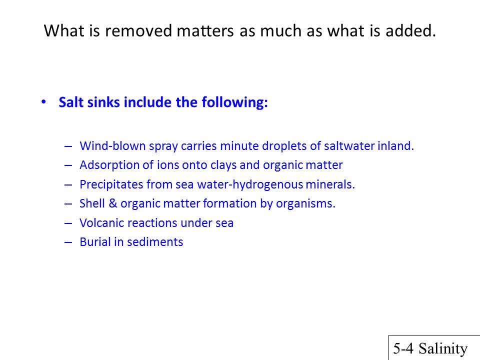 So if you have, if you have a- I don't know if you have- a big box of Quality Streets at Christmas, right, okay, and your mum comes on, keeps on topping it up with fresh Quality Streets, okay. the composition of what the you know how many, how many orange creams? 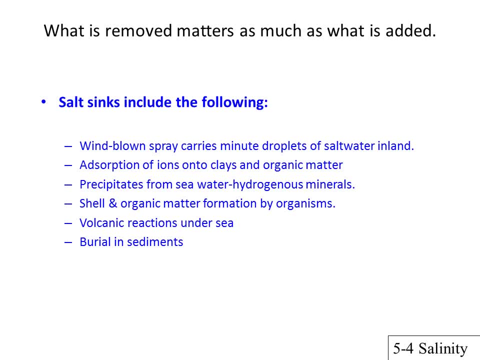 which are the nicest right. how many of those are left in that bucket is not just how many are added by your mum or other carer, but it's also how many you eat. so how many you take out, So that the input flux and the output flux are just as important. 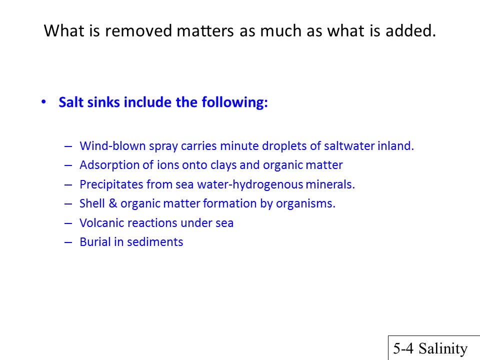 when determining what the composition, the composition of the, the of sea salt, is okay. So there are all these different ways that we can take stuff out, okay, So we talked a little bit so you can, you can take salts out of the ocean. 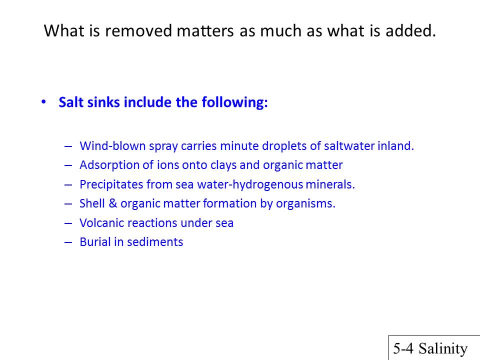 by forming sea spray, okay, And that sea spray blowing over the land, okay, And then that gets deposited on land and that removes every element that's in the ocean in that drop of spray. at the same rate, okay, Some elements absorb onto different minerals. 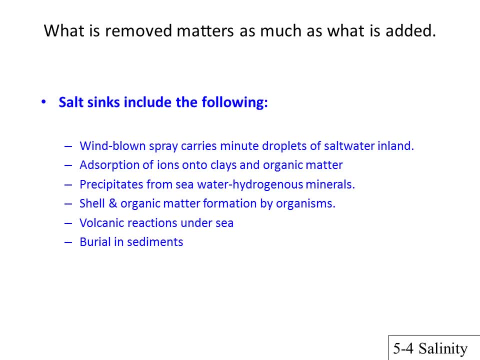 and that can be quite element specific. So particularly things like iron, manganese, they they can absorb onto stuff and be preferentially removed. So precipitates from seawater. I mean this is things like salt, So sea salt is made from evaporation of seawater. 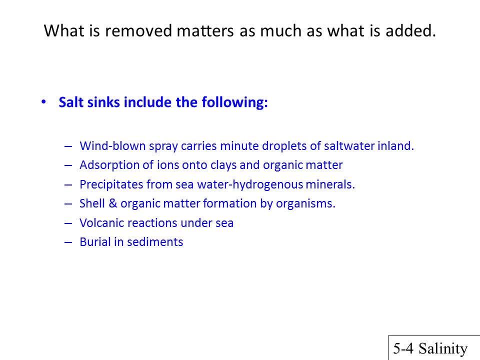 and in some places that happens naturally to such an extent that salt is removed from the ocean. okay, So that's one of the few ways that that salts are removed from the ocean, Forming shells and organic matter. So this is one of the one of the really major fluxes of stuff. 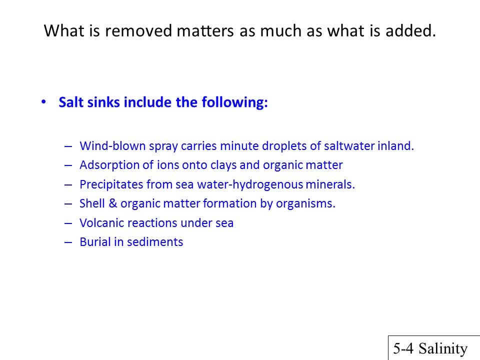 out from the ocean. So this is: if you're, if you're, if you're a little animal, or like a foraminifera or a coccolithophores, you build a shell. that shell is made of calcium carbonates. 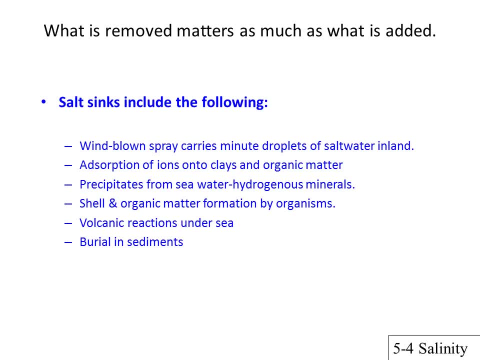 or strontium carbonates or opal, which is a form of silica That sinks, goes down to the seafloor. That's removed a little bit of calcium or a little bit of strontium out of the ocean. okay, 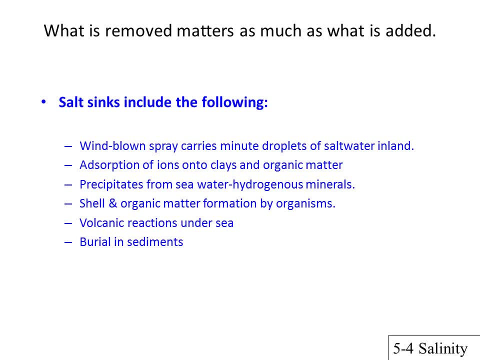 So there's a flux out of the ocean. by things making shells, You can volcanic reactions under the sea. that's similar to this absorption onto other minerals. So when water flows through a hot rock, some of the elements in the hot rock stick onto the, the, the hot rock. 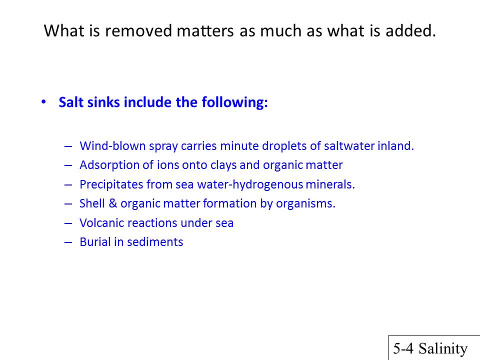 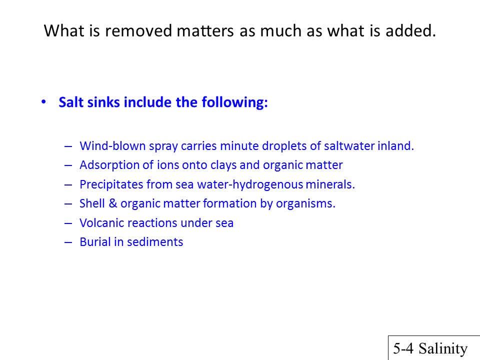 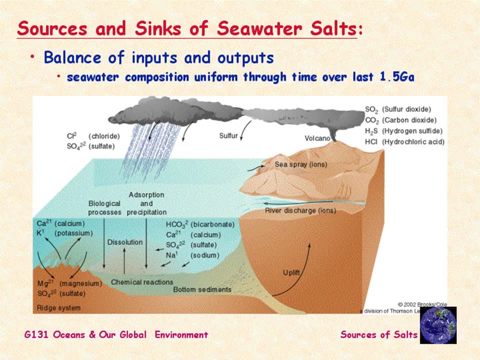 um, that's removed a little bit of seawater, therefore a little bit of salts, from the ocean, Okay. So all these different processes that that happen to remove stuff, Okay, and we can see, uh, a little diagram of some of these processes happening. 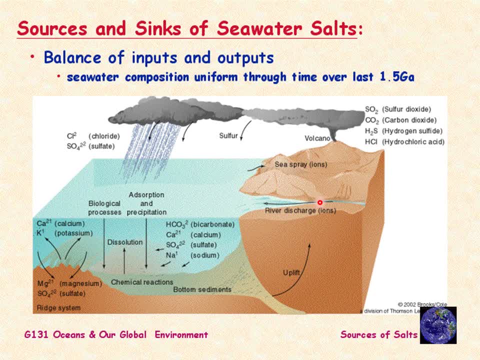 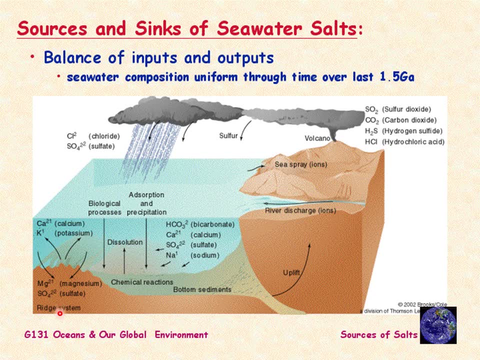 So you can see that, uh, ions are brought in from rivers and brought in from volcanoes, And there's an exchange of ions between seawater and rocks down here, So this tends to bring out leach calcium and potassium out from the, the rocks. 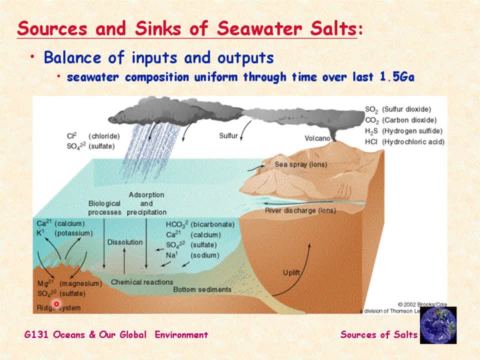 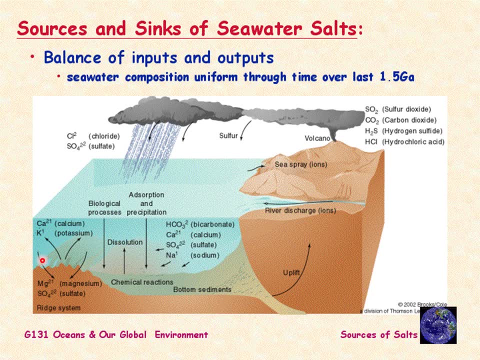 So when seawater circulates back through these rocks, magnesium and sulphate get stuck in the rocks. So basically it removes. it's like a filter removing ions from the the ocean, Okay, and then within the ocean, okay, so little beasties that that form shells will take up bicarbonate um calcium. 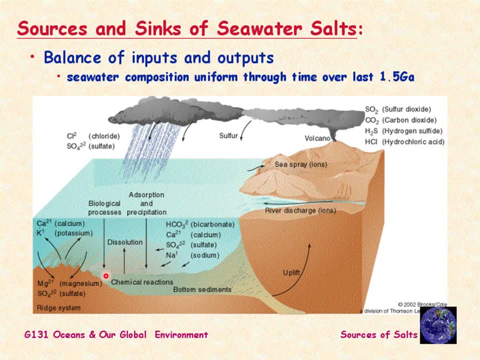 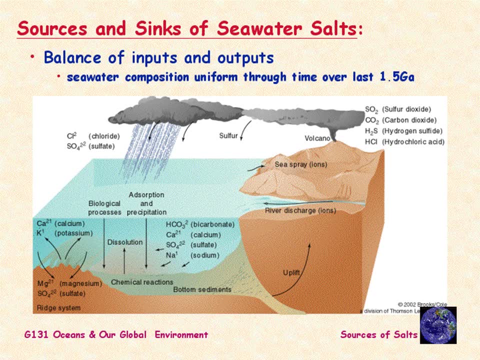 sulphate maybe, um, and they will sink down to the seafloor And be that those elements will be removed from the ocean And you'll also get removal from things like salt formation, Okay, And then burial, burial of sediments, you know, can remove stuff as well. 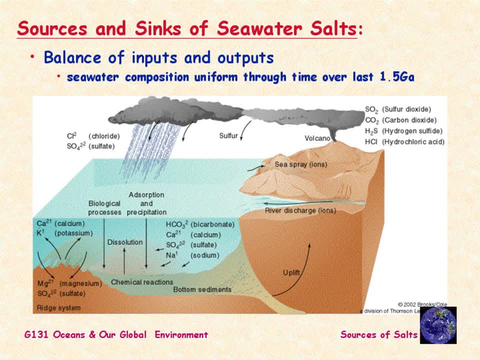 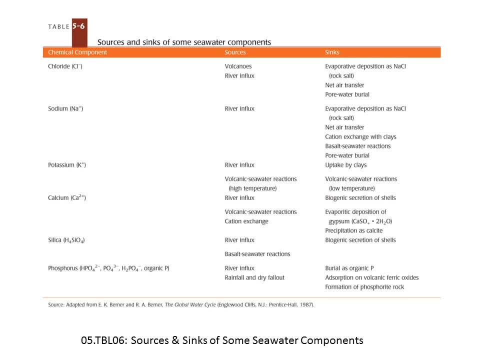 And they go into the rock cycle, which is very slow. Okay, and this is. this is a table of all that. I think you have the table. Do you have the table? Yeah, Somebody, one person nodded, so I'm assuming you all have the table. 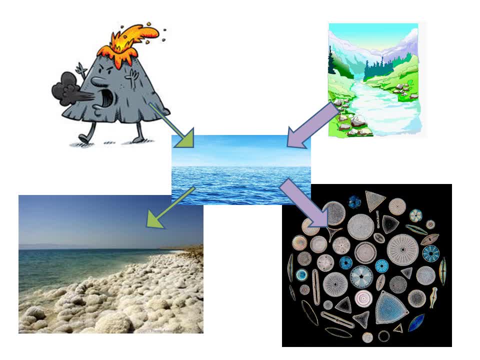 Right, so let me read the table. Um so uh, it's for different elements. these processes of addition and removal happen at different rates. Okay, and this is important for determining whether that element gets concentrated in sea salts. 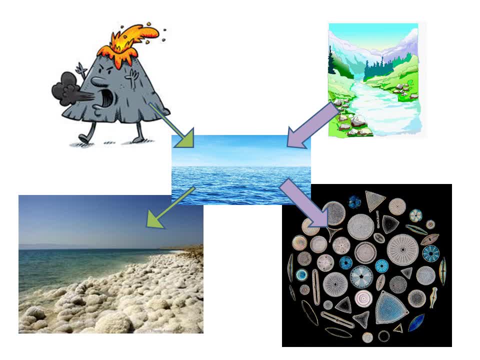 or gets preferentially removed. So in the case of something like chlorine that comes out of a volcano, It's actually quite a small flux, So that goes into the ocean And then it's removed by um sea salts, Okay, by salt formation, by evaporation of seawater. 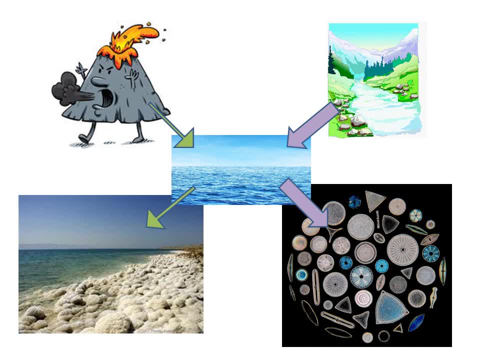 Okay, those are very small fluxes. So, um and the uh, chlorine is a very solid solution. Chlorine is a very soluble element, Okay, So that means that the ocean can hold a lot of it. Okay, Now the uh. this side over here. the other side is representing silicon. 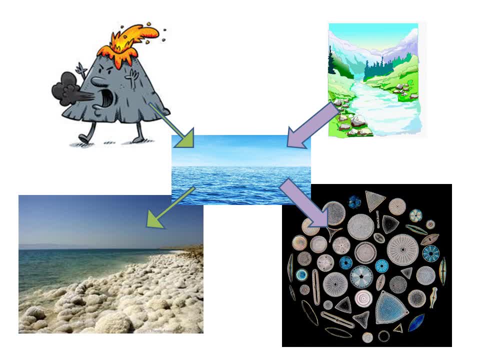 Now, if you remember from, the composition of, say, river water, rivers have got a lot of silicate in them, Okay, So the flux of silicon into the oceans is much larger than the flux of chlorine into the oceans. Okay, But the concentration of silicon in the oceans is much less. 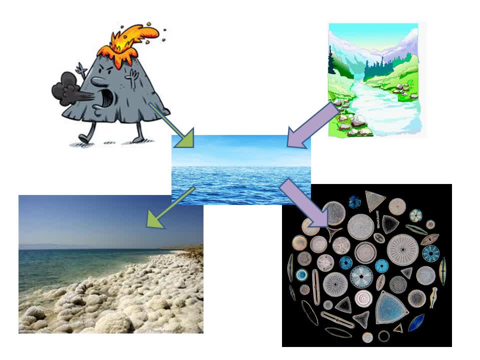 than the concentrations of chlorine, And the reason for that is because the output flux is also very large. Okay, So, even though you're adding silicon to the oceans, you're removing it before it can accumulate in the ocean basically, And in this case it's basically forming the shells of these things called diatoms. 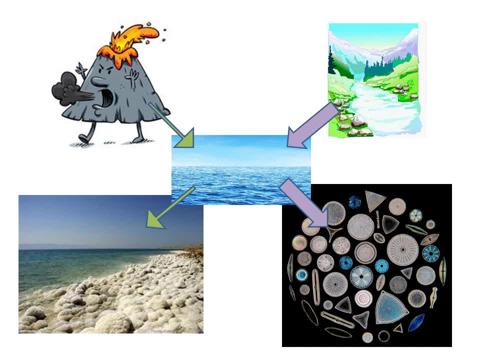 which are kind of, just like you know, the bottom rung of the- uh, the food chain. kind of ladder there If you- I mean if you get reincarnated- diatom is kind of like a you've been bad. 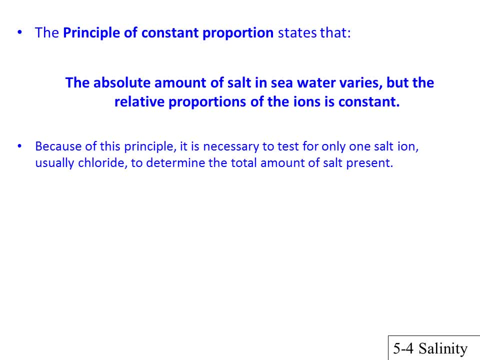 Um, but nice though. Um, okay, So we've kind of explained that, that different things are preferentially added or removed from seawater, And we're going to discuss this concept of, uh, constant proportionality, Okay, So we'll come back to this a little bit later. 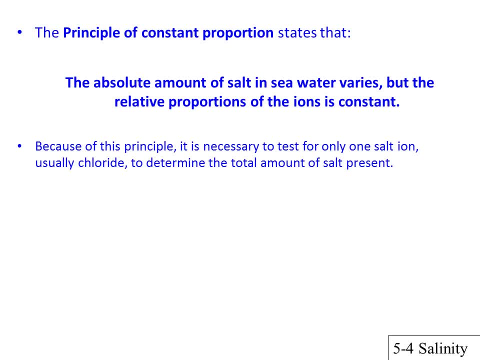 But basically for for some of the salts, so some of the salt elements, so sodium chlorine, um uh, potassium sulfur, um things like, um almost sometimes you can consider um calcium as as this as well. 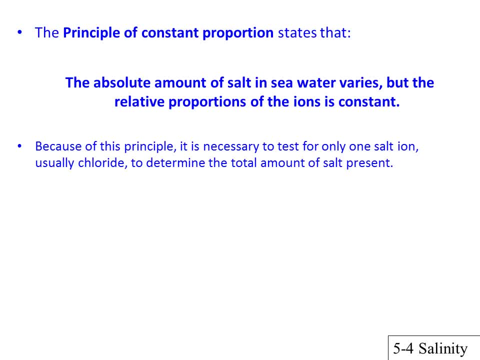 Because the fluxes into the ocean uh are very small compared to the amount of stuff that's in the ocean. the concentrations don't really change very much through time, Which means that the ratios of each of the different elements stays the same. 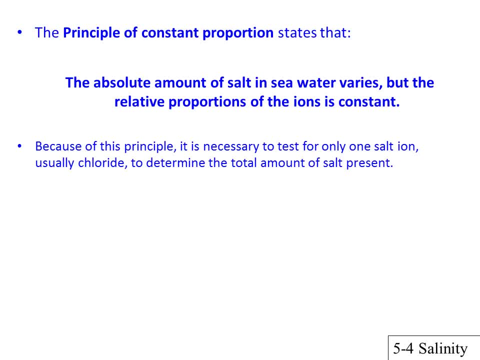 So, everywhere you go into the ocean, if you did the ratio of sodium to chlorine or potassium to sodium or sulfur to chlorine, that that ratio will always be the same, Okay, And this is very powerful because it- then it enables us to only measure. 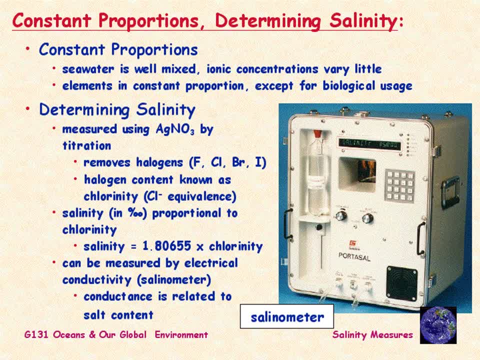 Okay, So the it. this is if we wanted to know how much of one thing there was, how much chlorine there was or how much sodium. we don't have to measure it, We can just measure one of the elements. 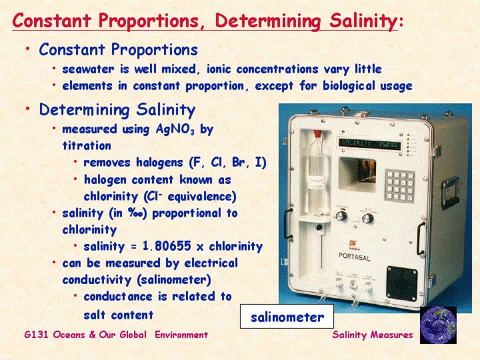 and that will tell us the concentration of all of the others that follow this: um constant of um, um constant ratio, Um thing, Okay, And this is. this is one of the machines that we use to measure um salinity of the water. 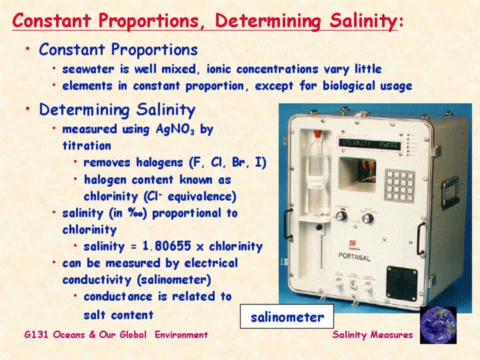 So there's this, this, I mean, back in the day, we, uh, we just measured um the total. uh, if we wanted to know how much salt was in the ocean, okay, you couldn't um. 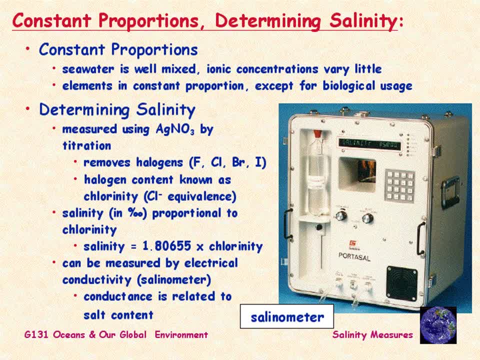 you couldn't take the seawater and dry it down and weigh what was left, because some of those salts would evaporate and then some of the some of the water wouldn't evaporate, so it would be held in hydrous minerals. 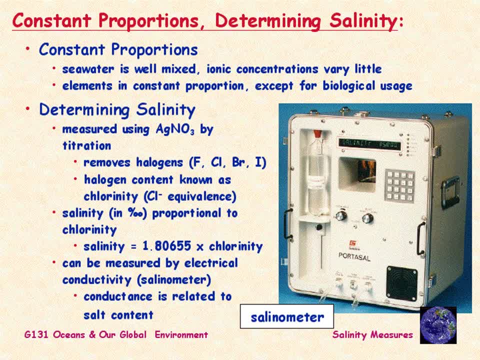 So instead of doing that, we basically we used this constant proportionality, where we just measured the amount of salt that was in the ocean, So we just measured the amount of chlorine, okay, And if we know the amount of chlorine, that means we know the amount of all of the other. 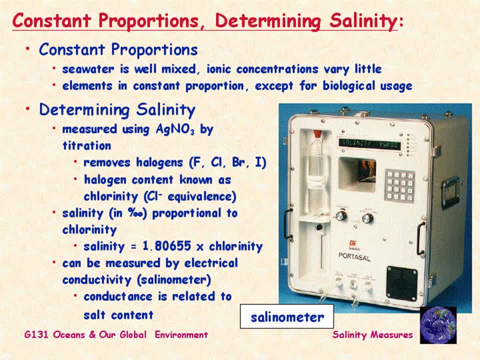 um, we would call them conservative or the constant proportional. okay, So the salinity would just be 1.8, something, something, something times the amount of chlorine. And we could do, and that's also. we also do it that way, because measuring the amount of chlorine is a way that 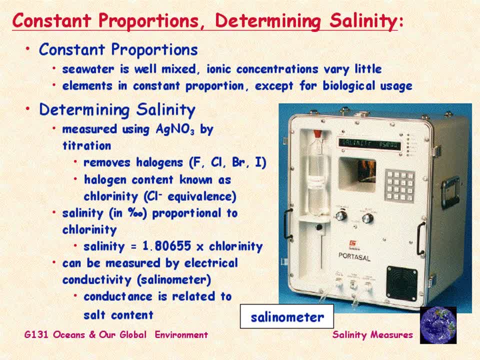 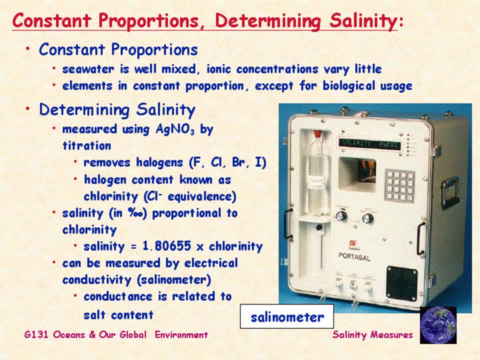 um is, is, is chemically very simple. simple in that you can basically just do a titration, Um, and there I mean there are the details of the titration, not the. you know the, the. 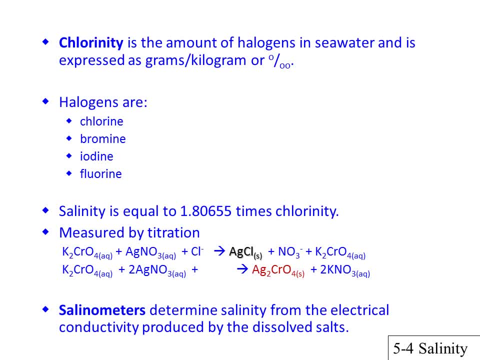 the but probably is very important, But, um, but we don't do that anymore. uh, because the amount of salt dissolved in uh in water is proportional to how conductive it is. Okay, So for pure water is almost a. 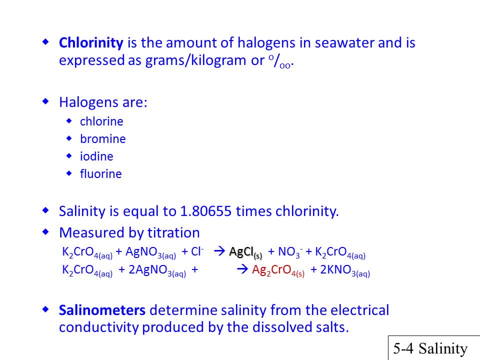 perfect insulator. Salty water. um, you know, don't drop in a toaster in a bath for salty water, because that would be bad. Um, so we basically just measured the conductivity of the water there and that tells us the salinity. 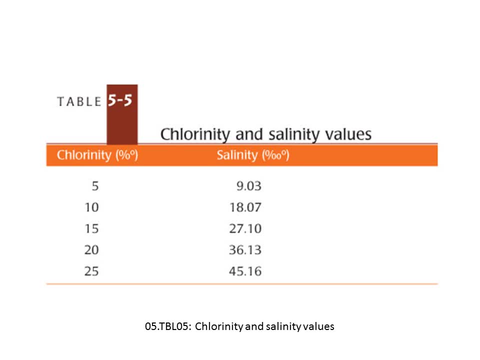 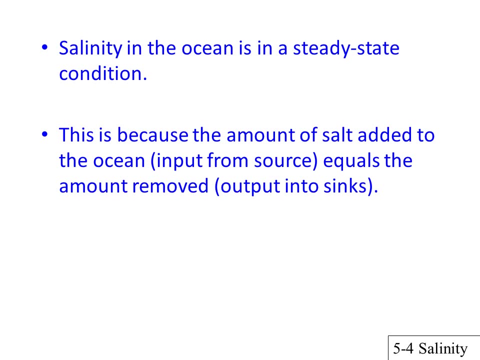 But that's just like a historical example. um, and these are basically so. i mean, this is, the amount of chlorine in the water is proportional to the amount of salinity. i mean, you can draw a graph if you want to, um, okay, so, um, i'm going to describe this. what do we mean by a steady state? why doesn't it change through time? 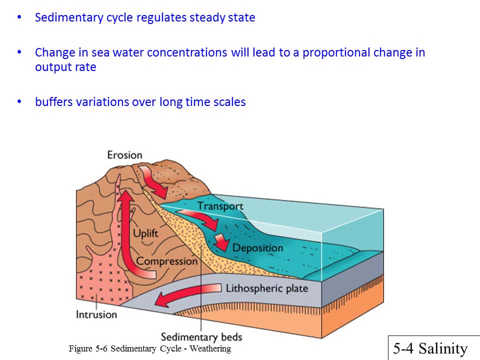 okay. so if we're looking at, um, uh, say the processes of addition and removal, okay. so if we've got, say, say, erosion, you know it could be erosion and volcanoes and hydrothermal, we just so erosion is adding salt and then we're removing salt or moving, say, chlorine by 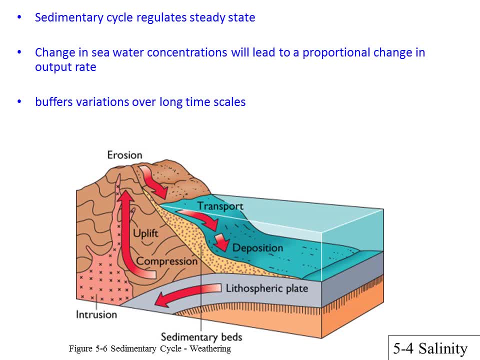 um, burying stuff in sediments, burying poor water in sediments, then subducting that so that the concentration of salt or sodium chloride or whatever element we're interested in that's remaining in the ocean, okay, is going to be a balance of those inputs and outputs. 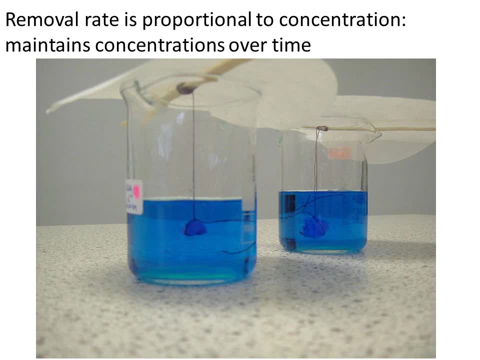 okay, so for almost all of the removal mechanisms, the rate at which you take something out of the ocean is related to how much stuff there is in the ocean. so the easiest way to think about this is from the example we've got here of basically just a simple chemical precipitate. okay, so the rate at which you form 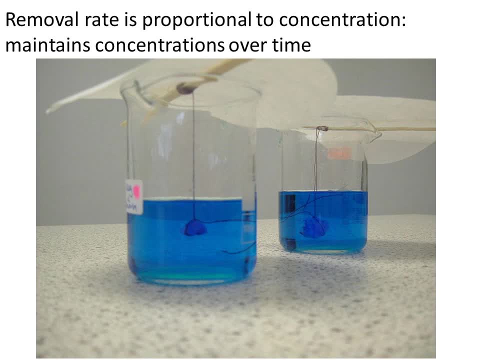 okay, this is this incident. you know you might have done this when you were seven. uh, um, but not eight. um, a, uh. this is a copper sulfate solution and you're precipitating out a little crystal of copper sulfate. okay, so the rate at which you can grow that crystal, the relative removal, 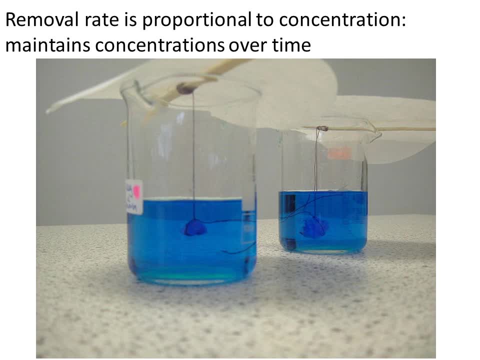 of copper from the solution- okay- is dependent on the concentration of the solution. okay. so if you have a very low concentration solution, the rate of removal will be low, okay. once you've got a high concentration, okay, the rate of removal will be faster, okay. so, because the rate of removal is dependent on the concentration of the solution, this kind of acts 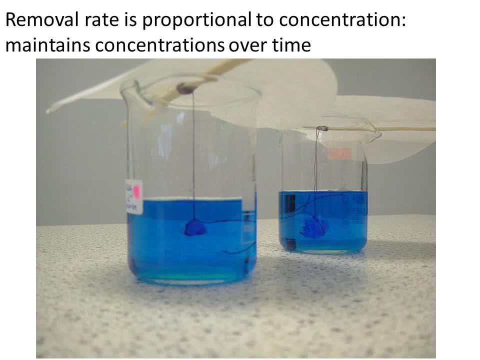 to moderate the concentration of stuff in solution. so if you have say, if we suddenly dumped a load of extra coper, or well, let's use the example of the ocean, right? so if we put loads of extra sodium chloride into the ocean, okay, that would increase the concentration of sodium chloride in the ocean. 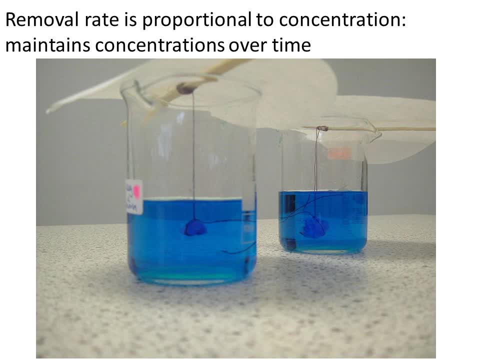 right adding more stuff in, but as soon as we've done that, okay, the removal rate would also go up. okay, because we've raised the concentration, so more salts will be precipitated out, okay, in regions of evaporation, and also more more salt will be removed in poor water. okay. 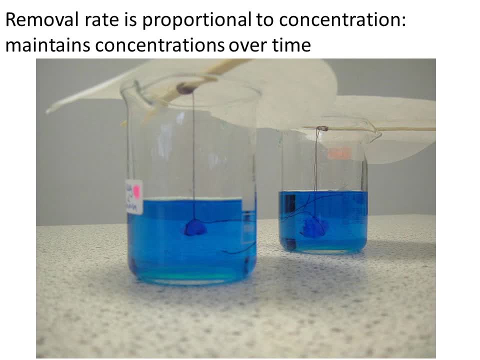 Because we're removing? because because the poor water will have a higher concentration of salt in it, And what that effectively means is that it moderates any changes in concentration. okay, So if we change the concentration, the remove, because the removal rate is dependent on that concentration. 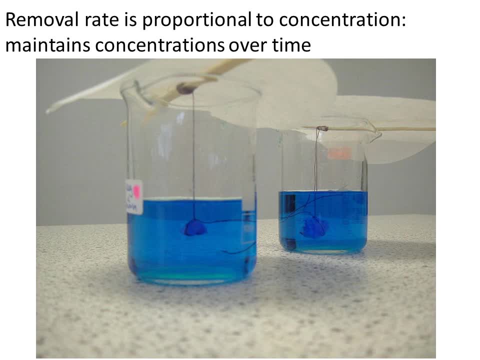 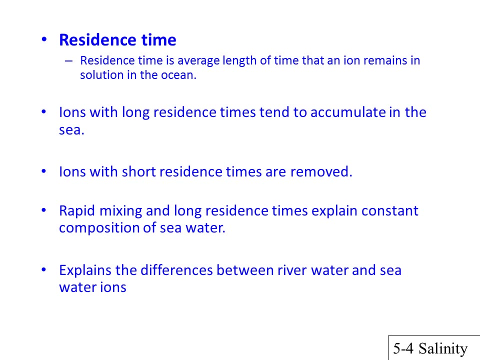 it will kind of act to, to, to, to smooth out the any changes. So concentrations of some of these very, very soluble salts tend to stay constant through time. okay, Now we're going to go on and talk a little about this concept called residence time. 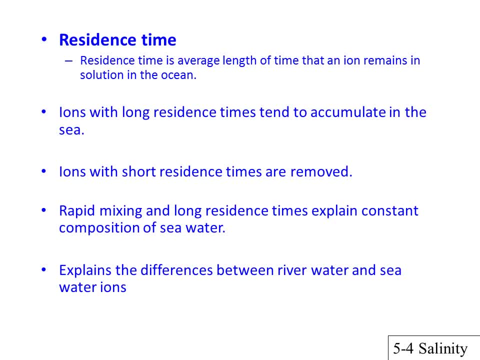 So residence time is is basically the average amount of time an an atom of that salt, that element, is in the ocean or in any reservoir. okay, And it's quite a useful property to know, Because if you can calculate the residence time, you can predict how something might change through time. okay. 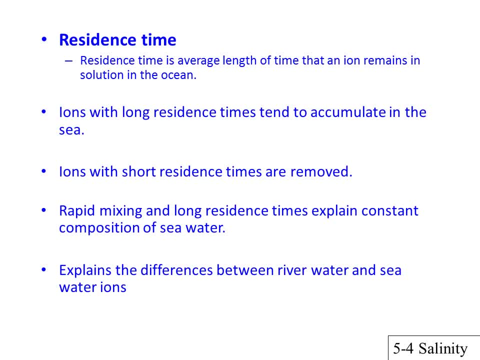 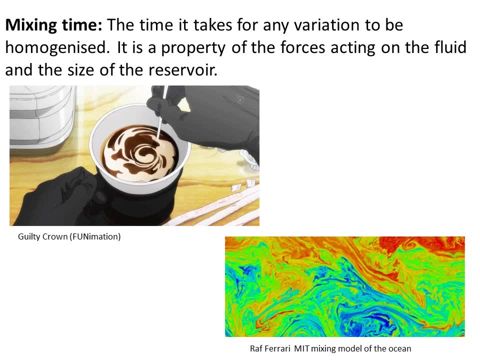 You might predict whether it's possible that that thing has changed or not. okay, So, but before we talk about residence time, I just thought I'd put this up here and talk a little about mixing time. So there's a concept of residence time, which is about how long something stays in the solution. 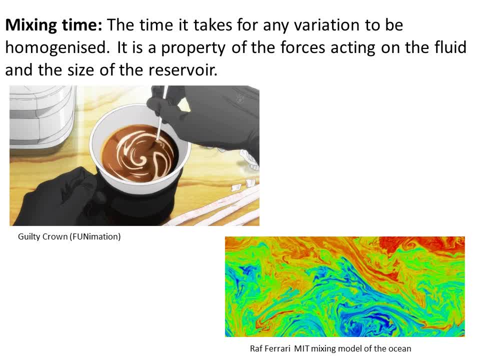 And there's this concept called mixing time. Can you stop whizzing? Okay, there's a concept about mixing time which is similar But different. So the mixing time is the amount of time it takes for any variation in your fluid to become evened out. okay, 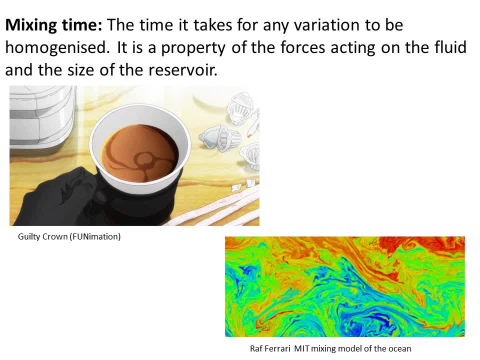 So the mixing time of, say, a cup of water or a cup of tea in this kind of like slightly sketchy Japanese anime thingy here is: it's quite short, It doesn't take very long okay. 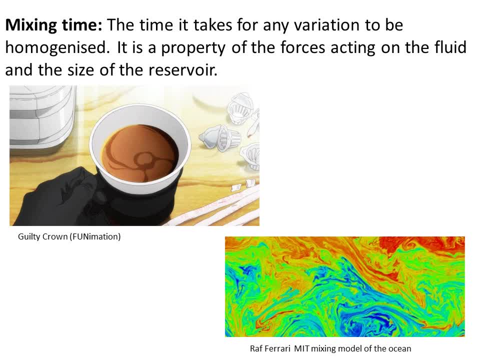 But it's a property of the physical dynamics of that cup of water. So A cup of a cup of coffee. if we had two cups of coffee, okay, add milk into them. they're chemically identical. But if we stir one, okay, it'll have a shorter mixing time than the other one. okay. 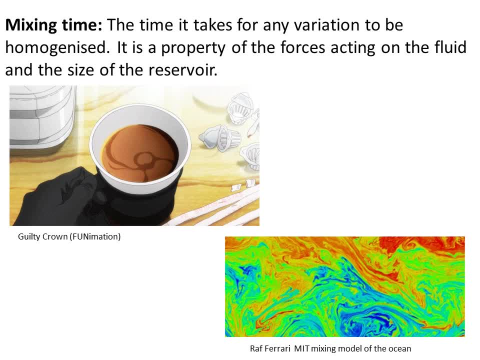 So mixing time is a property of the physical dynamics of the thing, okay, Of the reservoir, not of its chemistry, okay, And this, I mean this, these kind of things, these swirly patterns, happen in the ocean as well. 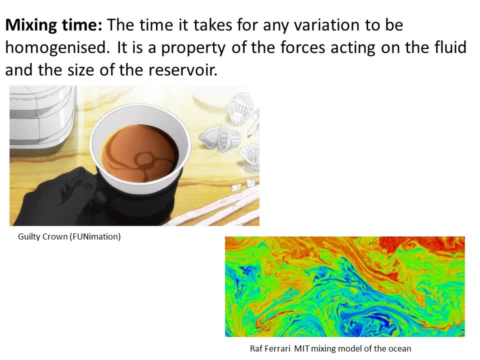 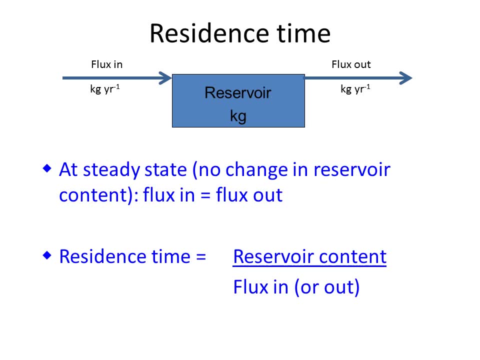 I guess you might have seen stuff at the beginning of the lecture. there were some swirly patterns as well. okay, So mixing time is about mixing. Okay, so the residence time is different. Okay, so with residence time, we're talking about what is the? basically the relative sizes of the fluxes in and out of our reservoir. okay, 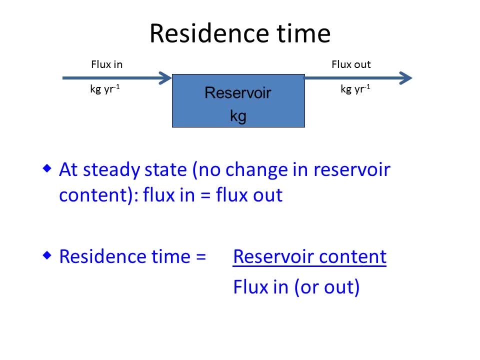 Relative to the amount of stuff in the reservoir. okay, So when we calculate these things, we assume a steady state. Okay, so we'll come on to a little bit what that means in a bit. But basically, if you want to calculate a residence time, the flux in and the flux out, you have to assume that they're the same, okay. 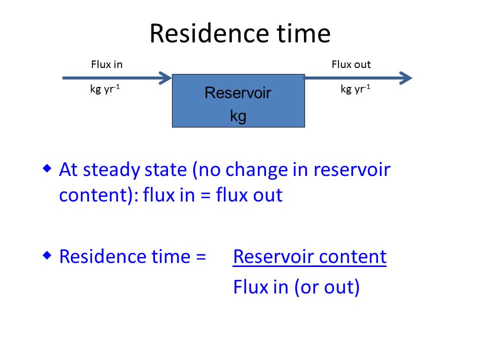 And that means that the concentration in the reservoir is not changing. okay, And there's the equation to work it out very super simple: residence time, reservoir content divided by flux. You can work out the units from that in your own time, and the units are, of course, time: residence time. 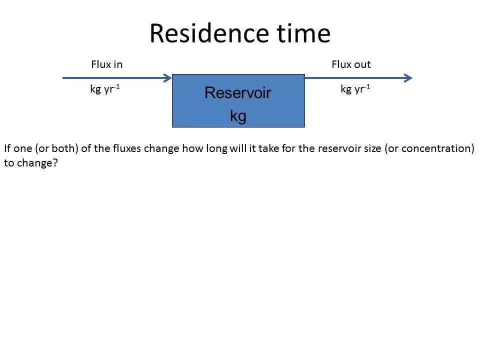 Okay, so let's see what happens If one of these fluxes were to change. okay, it's basically how long would it take for the concentration or the amount of stuff in the reservoir to change? So if, for instance, we increased the flux of stuff into the reservoir and this stuff can be anything, okay, 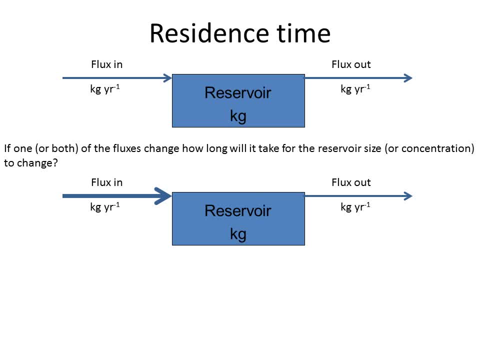 It could be water itself, or it could be salt, it could be a nutrient- okay, It could be anything, okay. So if we've increased the flux in, So if we, if we- I guess this is a graph of time- against amount of stuff in our reservoir, cycle time. 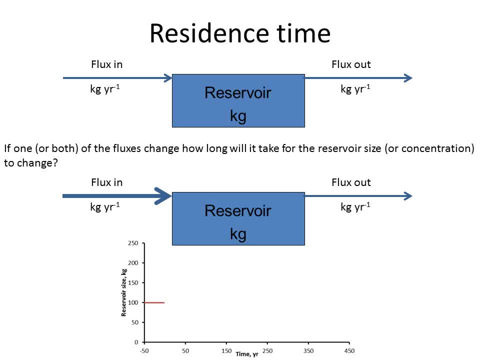 So start out with very constant case at the top, and then and then, and then, over time, The, the concentration or the amount of stuff in the reservoir will start to increase. okay, But as the concentration increases, the flux out should also increase, because the flux out is dependent on the concentration. 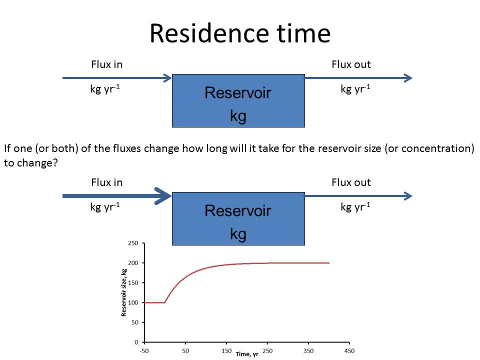 Okay, so you should then eventually reach a state where the concentration is not continuously going up, because the flux out will have gone up. Okay, I should have made that arrow a little bit bigger. Okay, so that's bigger. So you start out in a, in a situation where you're in steady state with the amount the flux in equals the flux out. okay, 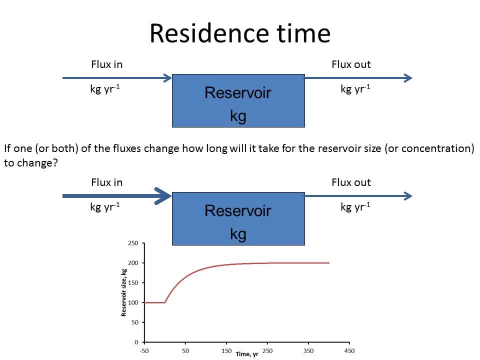 And then you perturb that by making the fluxes different sizes, But then, because the flux out is dependent on concentration, they will tend to to a situation where the fluxes are equal again. okay, But in this case the concentration is now higher. 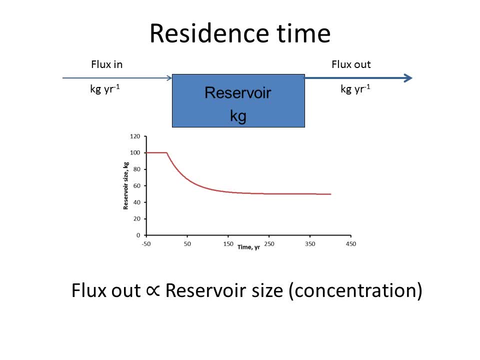 Okay, so you could do the similar kind of thing here. So okay, In this time I've just made the flux out bigger, So you might be able to see that arrow is slightly, slightly bigger. In this case, by increasing the flux out, the concentration goes down, okay. 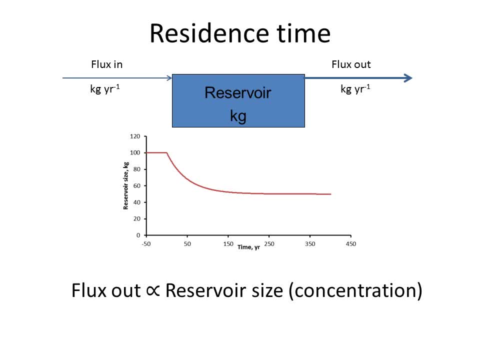 But as the concentration goes down, the flux out will then also reduce, as because it's related to the concentration in the reservoir. Okay, so the, the flux is proportional to reservoir size and that's what moderates the, the change in the, the reservoir size. 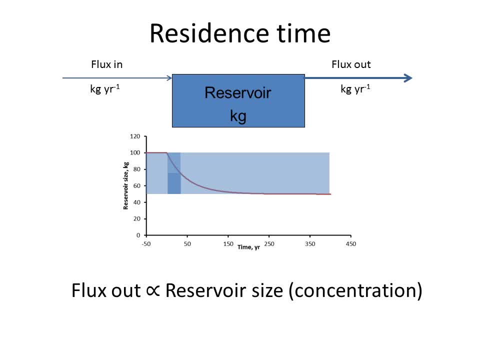 Okay. so if we look at some of the the time scales of these changes now, so if we look this much, so the amount, the amount of change has gone from 50, gone from a reservoir size of, say, 100 kilograms or 100 beans or 100 busloads or whatever unit you're, you're measuring your stuff in. it's gone down to 50, okay. 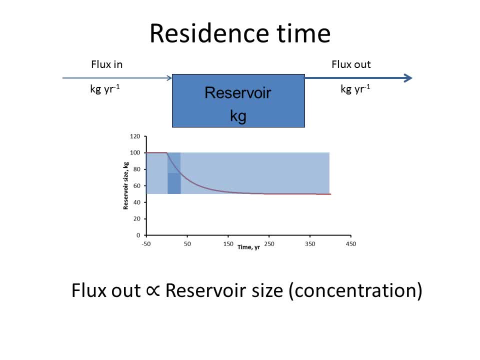 So we could look at the time it takes to go to 75, so half of that difference, okay, And that you might be familiar with the concept of half-life From radioactivity or whatnot. okay, So we could describe the residence time in terms of the, the the half-life of that change, okay. 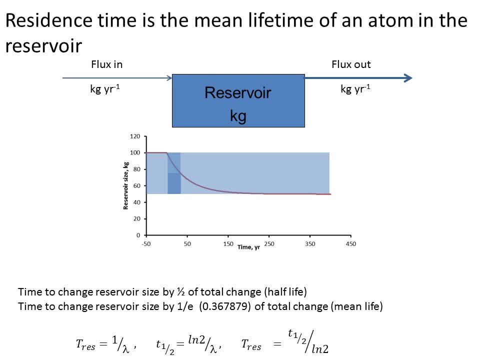 So we could do that, but what we actually do is we use um, this term called the mean life, okay, Which is which is related to the half-life, but instead of the time it takes to reduce to half, it's the time it takes to reduce to 1 over e, which is like one of these irrational numbers. 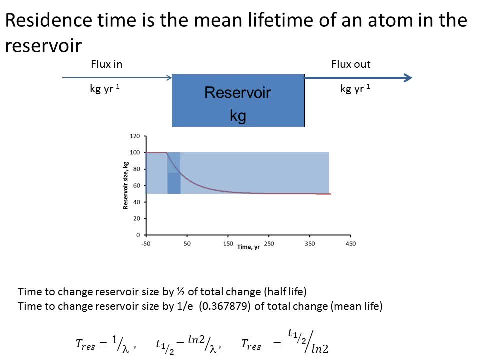 Um, but Uh, it turns out that that's quite useful because instead of the half-life being related here to log 2 over the decay constant, okay, So the the residence time, if we use this 1 over e, is actually just 1 over the um decay constant. 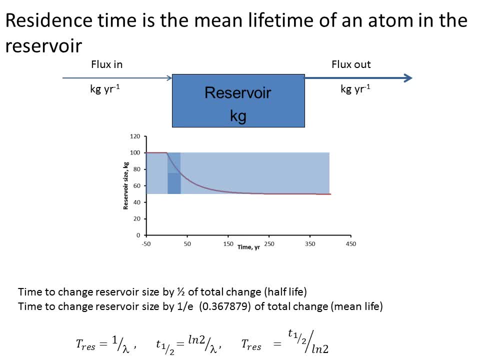 So it's basically a mathematically simpler way of describing how fast it takes something to change if it's following this exponential um decay thingy. So the um, so we actually define it as that. In this case it takes 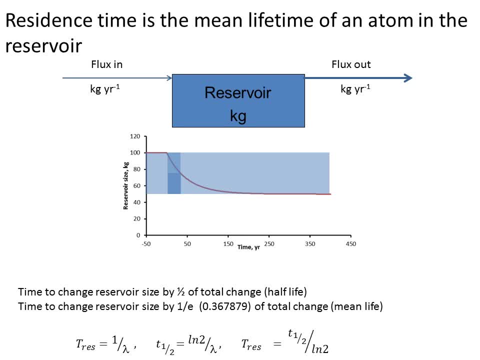 50 years. okay, to uh get down to this 1 over e or 0.3, something, something, something, something, something, uh of the total change, okay, So uh, you don't need to know all of this stuff down here, but basically, uh, that number t res the, the residence time or the reservoir time. is the flux in or the flux out, if it's at steady state, divided by the reservoir size. 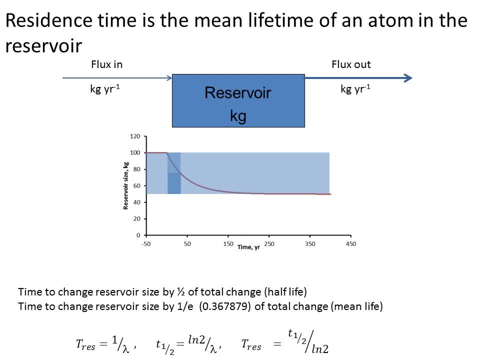 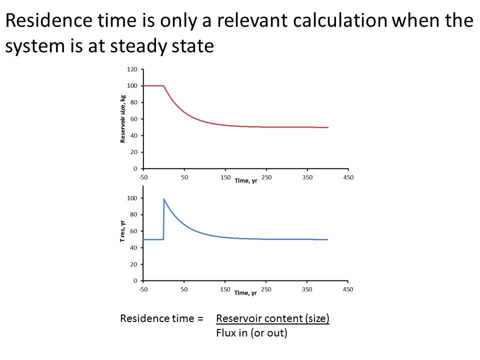 Okay, no, the reservoir size divided by the flux, so, um. and that turns out to follow this equation here. okay, So that's why we use that one and not the half-life one. Um, so, if we do that calculation. so this is the same example again. 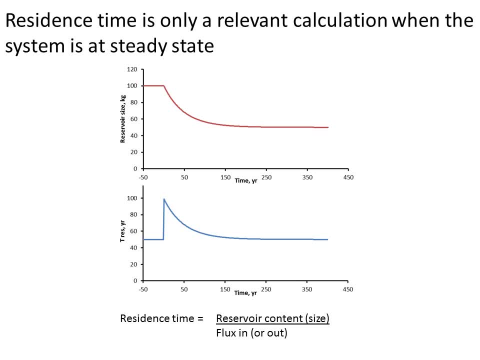 Uh, so we've reduced the flux out, so the concentration reduces over time. So I've calculated the residence time uh, at the beginning, okay, That's 50 years uh, and then as soon as we change something, the flux in. 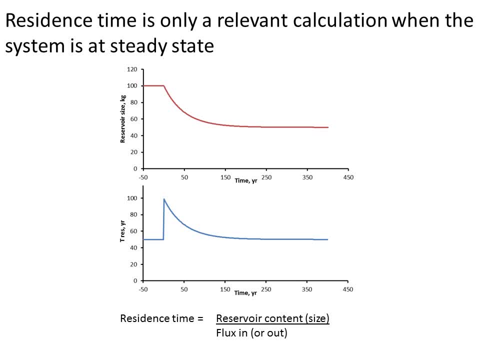 It doesn't equal the flux out. okay, So the although I've got the the residence time spiking up here, that's because I've I've the reservoir amounts have stayed the same, but I'm using the flux out okay. 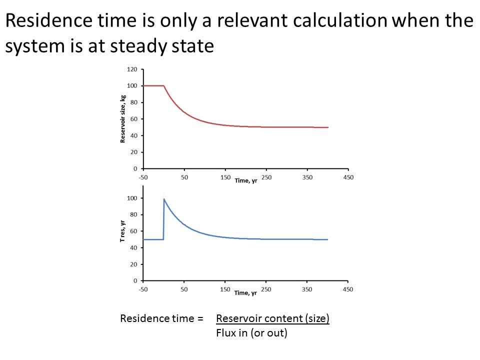 To calculate the residence time, uh, and I get a much bigger value because the flux out is reduced. Okay, So that's not, um, that's basically that's, that's, it's, it's, it's meaningless that the calculation 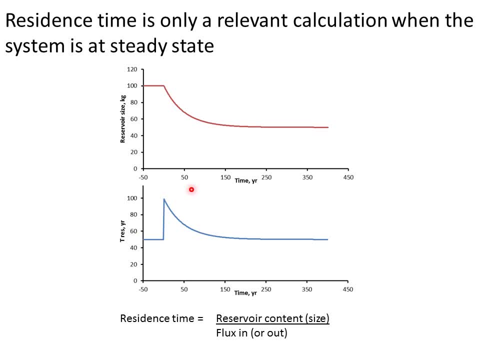 During in this, hang on. let me show you the little. This part: here, the calculation of the residence time is meaningless because the flux in does not equal the flux out. okay, But over time, over time, the um, the, the, the residence time will approach this equilibrium value where the flux in equals the flux out. 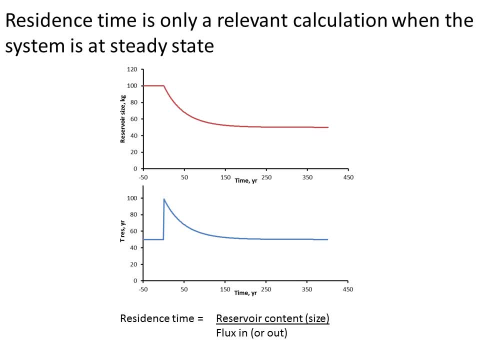 I should point out that, um, the Excel file that I've used to create these, uh, these graphs, um, I've popped it on learn um, and it like draws the graphs and stuff like that. So you can have a play with that, you know using. 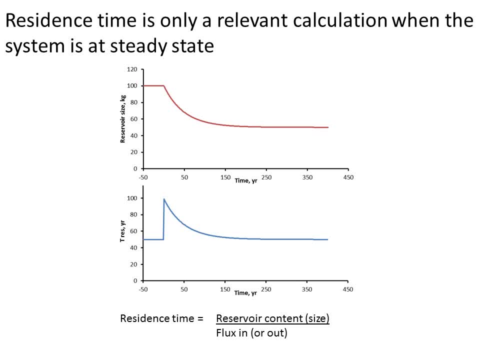 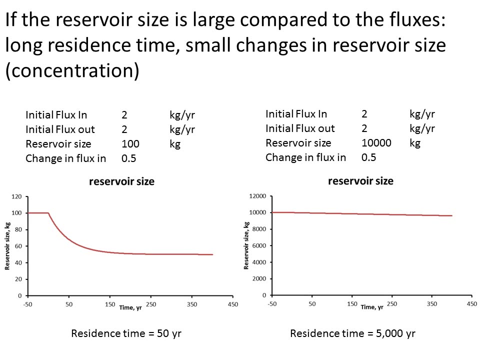 Changing fluxes in, changing fluxes out, changing reservoir sizes, to see what um, to see how it affects what happens with terms of how fast things can change their concentration, Um, and just an example of that. So if I start out with an initial flux of two, the flux out equals two. 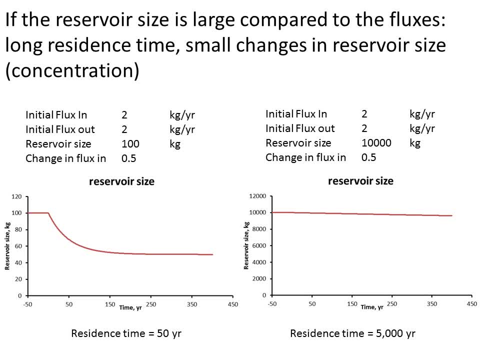 So we start in a steady state. We've got a reservoir size of 100 kilograms In in a, in, in in a 19-안� 귭 zwkw, zwkw, zwkw, zwkw, frying Me OFF CSains. 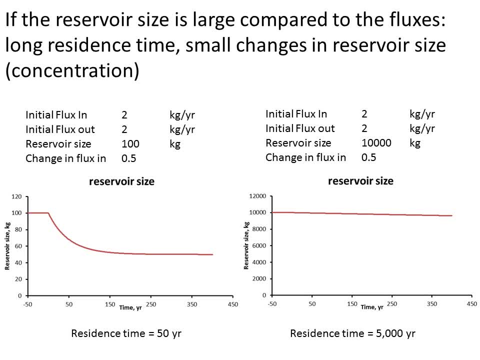 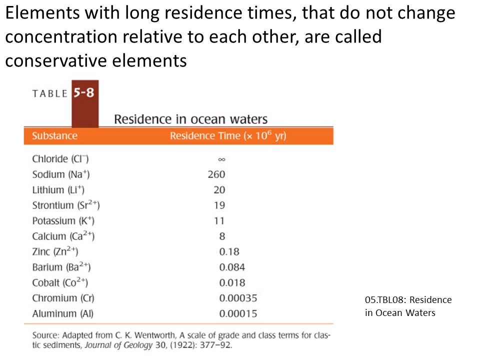 me OFF, free, free, free, free, free. you damn near okay. so. so what about that thing anyway? so, the elements with long residence times: okay. so if you've got a very long residence time, that means your concentration is very unlikely to change through time, which is why the elements 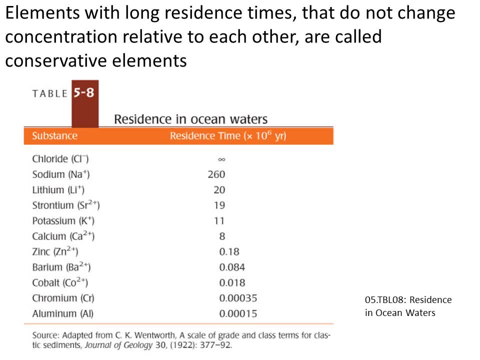 like chlorine, sodium, lithium, strontium, potassium. it's why we call those conservative elements, because their concentrations relative to each other are not going to change by much. okay, so the only way that you can really change the concentrations of those elements in the ocean is by 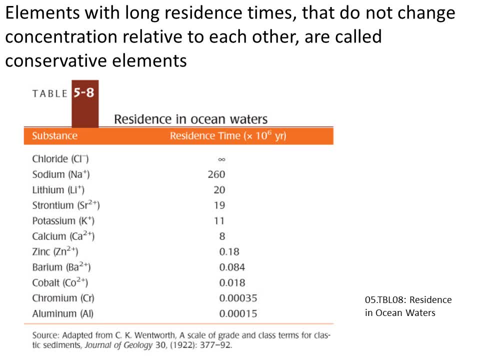 taking water out of the ocean or adding water. okay, so if you did that, so if you took water out of the ocean, the ocean would get more salty, the concentrations would go up, but the ratios, the amounts of those relative to each other, would stay constant. okay, and you can see from this that 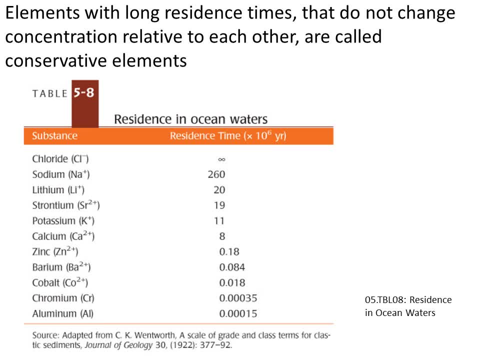 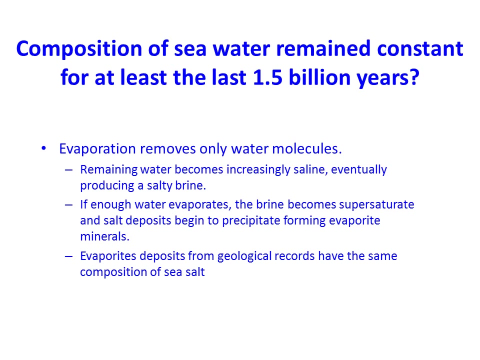 basically, the chlorine has essentially got an infinite residence time because there's so much of it dissolved in the ocean. fluxes are so small that essentially it will never change the amount of sodium chlorine in the ocean. okay, so composition of the ocean is basically so the amount that the types of salts in the ocean have been the same. 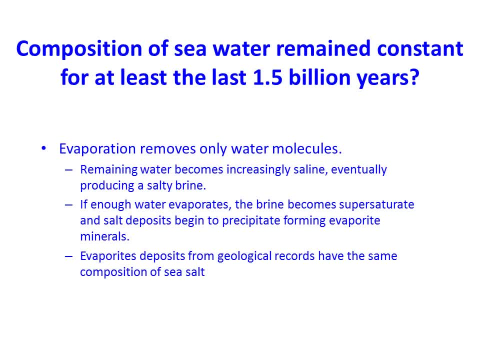 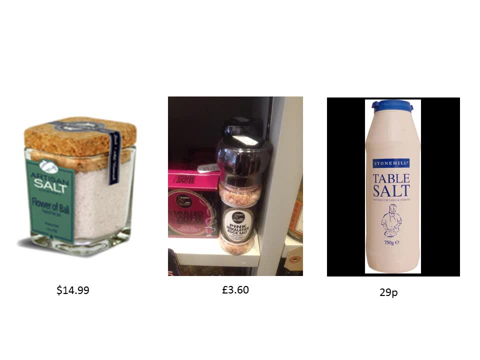 over all, of almost all of geological history, or at least the interesting parts of geological history, which which means that all of these different kinds of salts which ultimately come from the ocean, so this artisan salt that Americans buy for $15- if you get a Stockbridge you can buy. 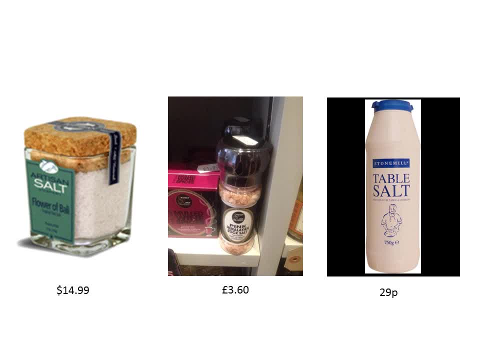 Himalayan pink rock salt, which ultimately comes from the ocean, probably 20, 30 million years ago. there's 3 pounds, 60 on that, or you can go to Lidl and you can get 29p salt. okay, it's the same salt, okay. so if you want salt, 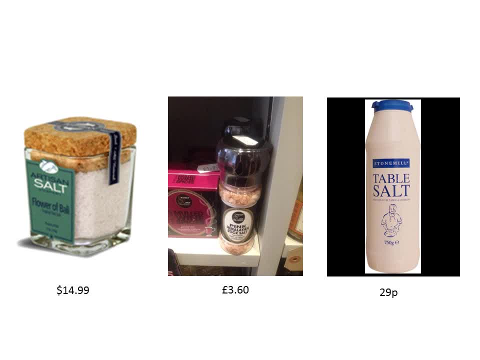 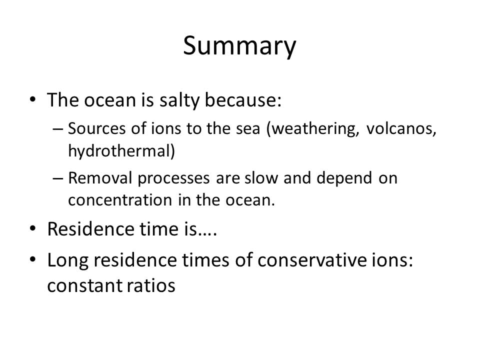 I'm not suggesting you have a high salt diet, but buy the Lidl salt because it's chemically the same ish, okay. so some kind of reminders of what we've done today. so the ocean is salty, but it's not so salty- salty because the fluxes in- okay, are only really in and we don't. we recycle the water. 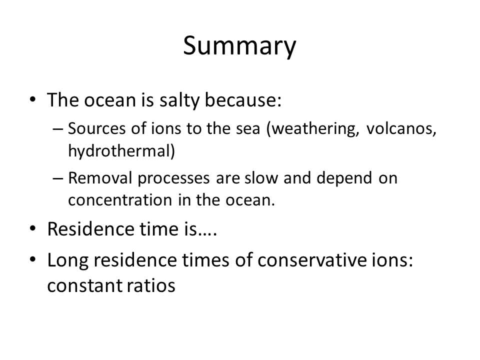 but not the salts. But the fluxes in are different compositions to what's in the ocean and that's because we have these different removal mechanisms that affect different elements specific. So, for instance, the formation of calcium carbonate shells removes only calcium from the ocean, and 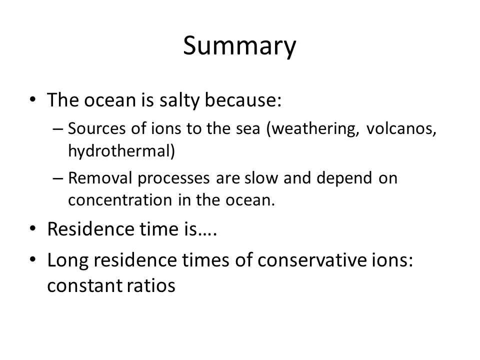 doesn't remove silicon or sodium, okay, whereas different. so the different processes cause there to be different- determine what the composition of salt is in the ocean. The residence time: okay. so I put the residence time is okay, but you should hopefully go back through all that stuff. 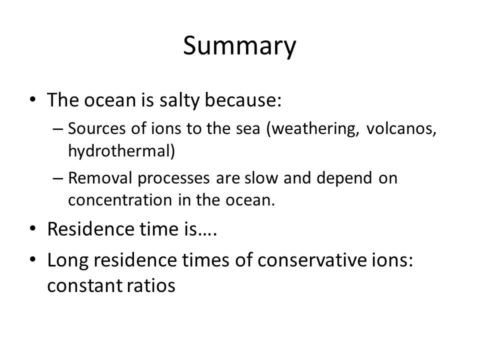 and figure out the difference between what a mixing time is and what a residence time is, and why. having a long residence time means that the composition of something doesn't change, and having a short residence time means that, basically, if you've got a residence time that is shorter than the 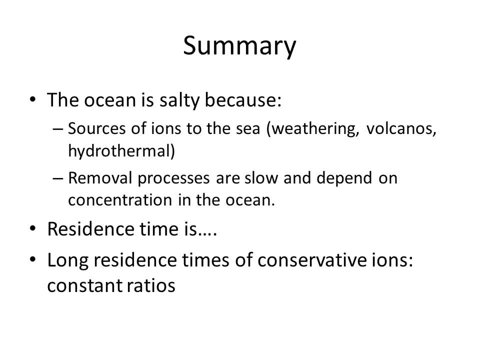 mixing time. I didn't really explain this. so if your residence time is longer than the mixing time, okay, that means so, for instance, the ocean: for sodium or chlorine mixing time of the ocean is about 2,000 years. the residence time of chlorine is like super long, so that 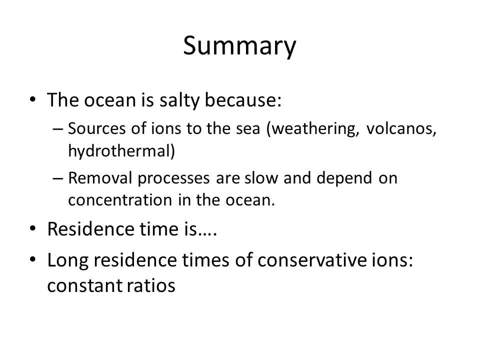 means that it's completely different. So, for instance, if you've got a residence time of chlorine, okay, that means that it's completely mixed for chlorine or sodium, okay. so the concentration will be the same everywhere. but for the things that have got a very short 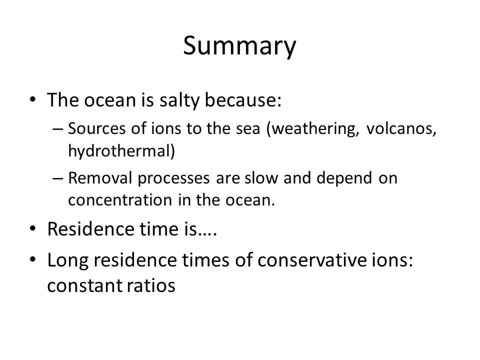 residence time. okay, so that may be silicon or some of the nutrients that are removed very rapidly, so their concentrations are very low relative to the fluxes. okay, that means that the ocean hasn't had time to mix out all of that variability in concentration. 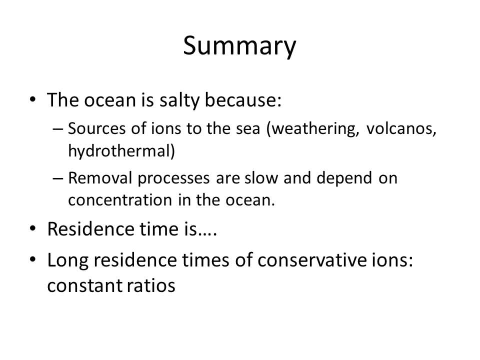 okay, which means that if you go and measure the concentration of different elements that have short residence times, is that you will find that the ocean is quite variable. Some places will have a lot of nitrate, some places will have no nitrate, some places will have 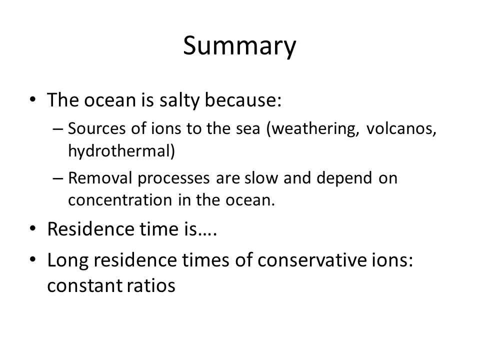 lots of silicon, some none. some will have no iron, some will have lots of iron- okay, and we'll come on and talk about those variations next week after Simon's done his stuff, okay, Okay, so have a look at the stuff I've learned. it's hopefully useful and I will see you. 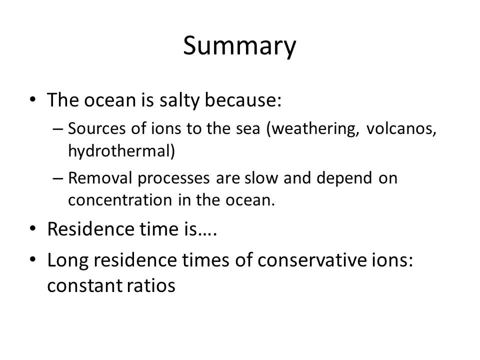 all next week, Thank you.